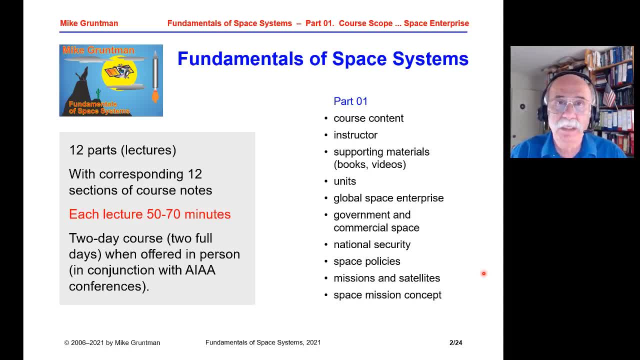 a two-day course, two full days, eight or nine hours per day, and this course is typically offered in conjunction with AIAA's conferences. Today, in this lecture, we will start with the course notes: Fundamentals of Space Systems. 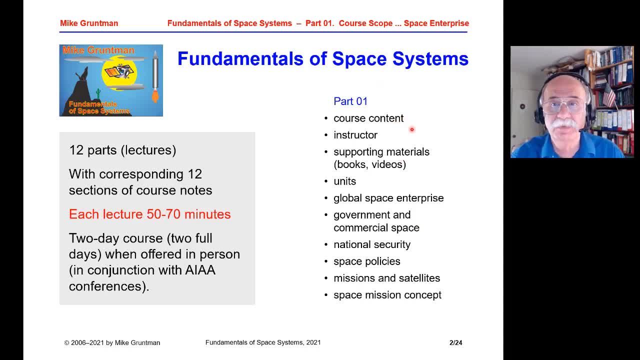 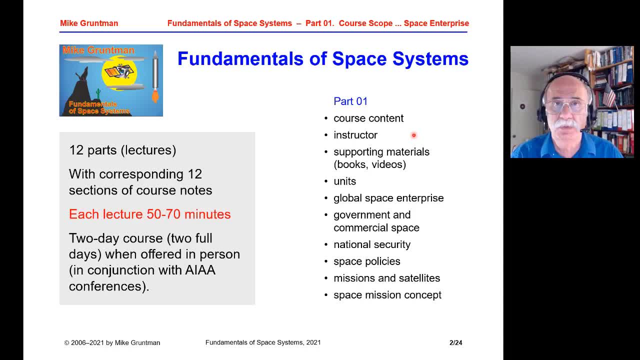 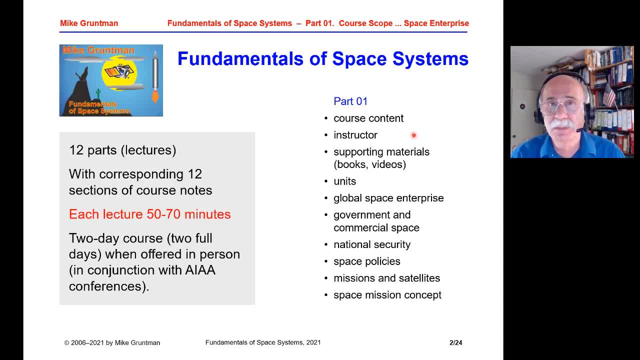 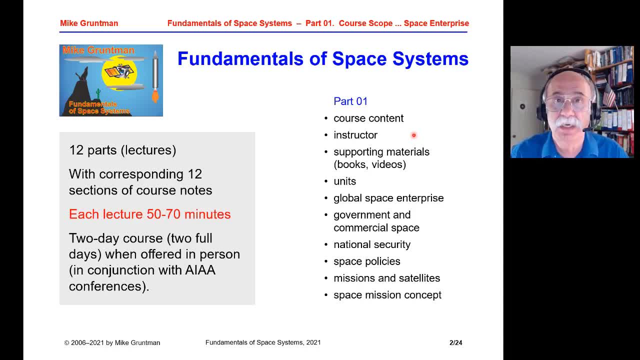 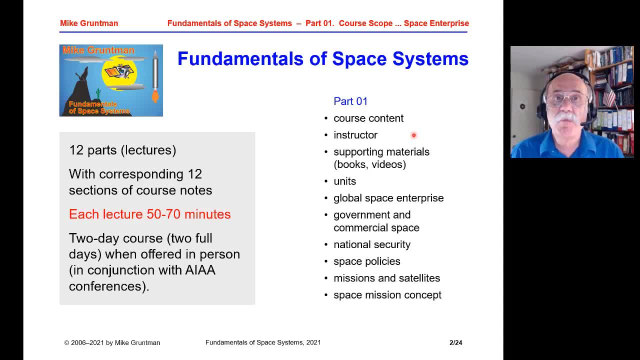 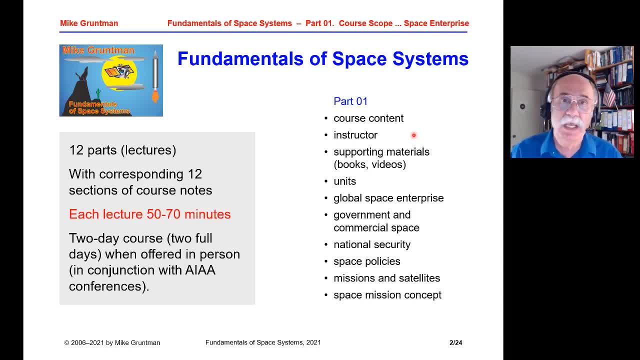 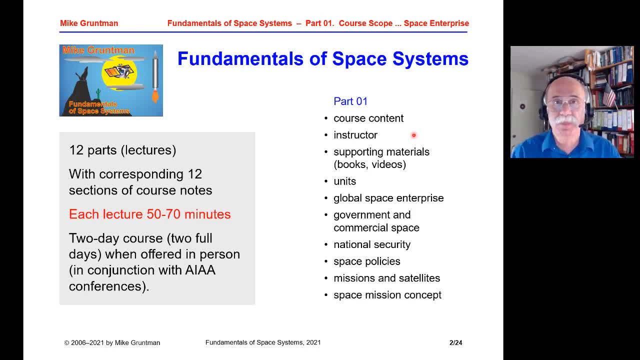 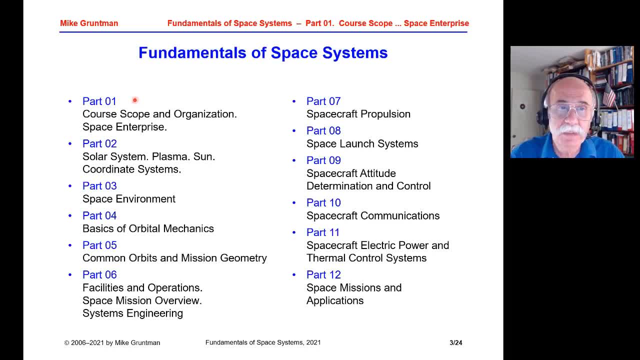 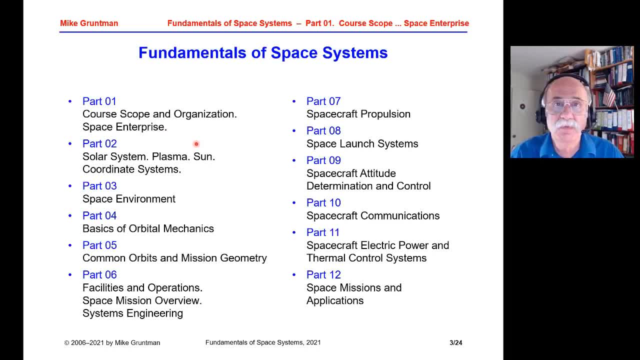 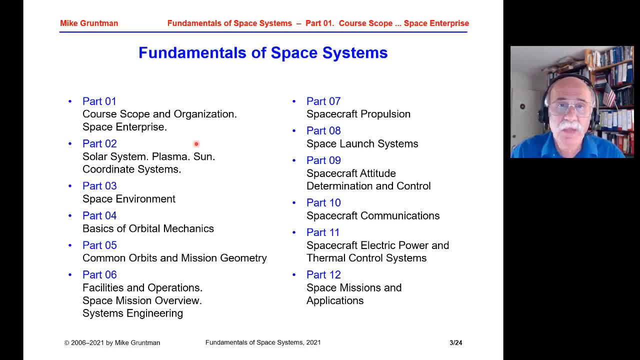 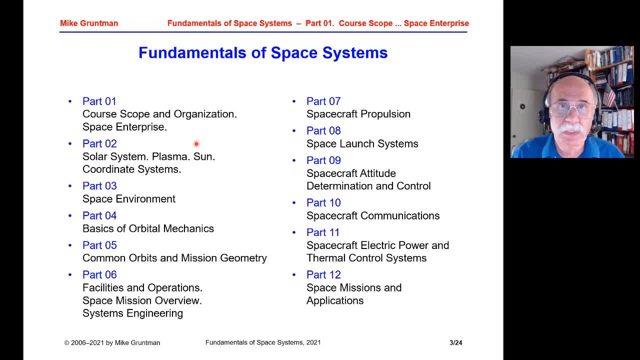 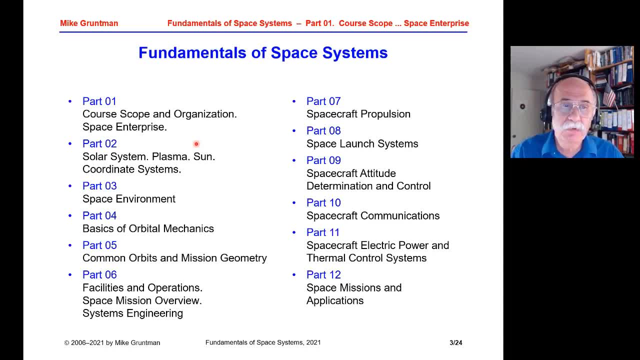 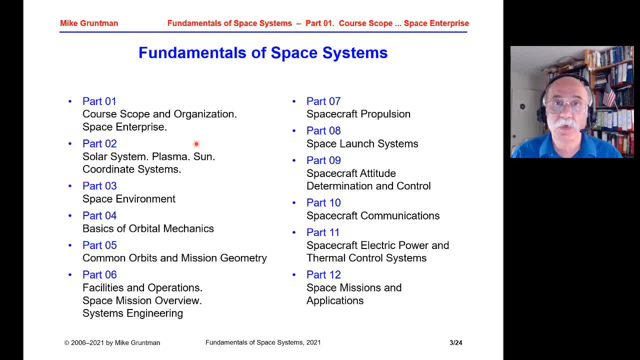 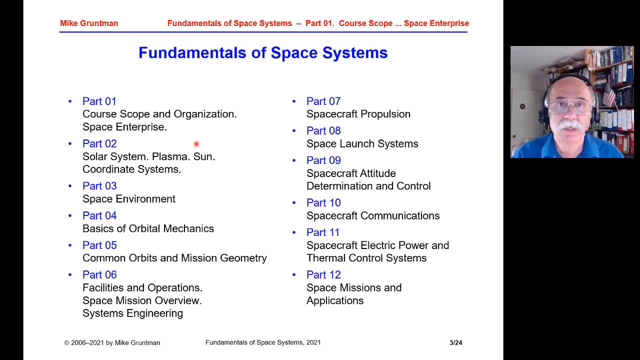 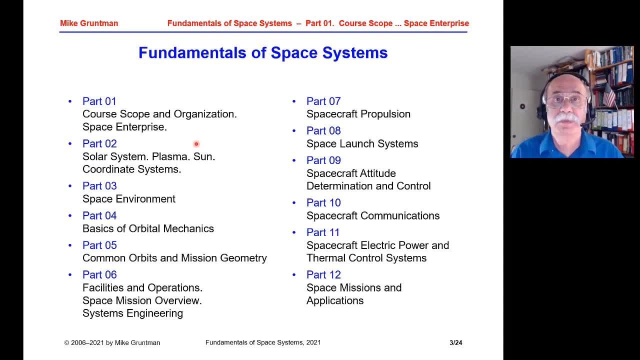 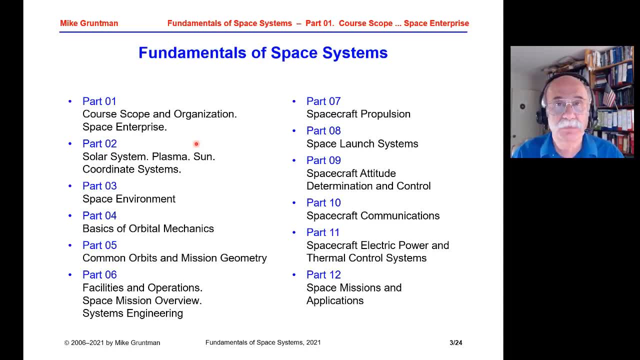 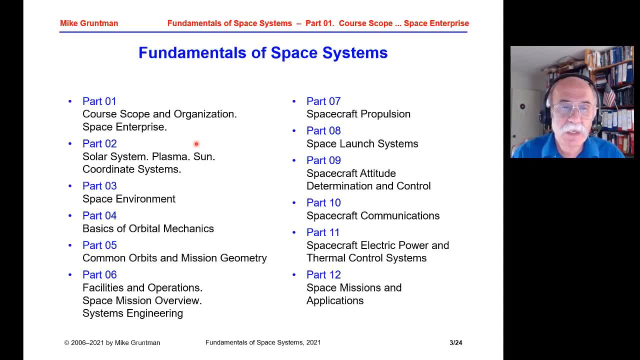 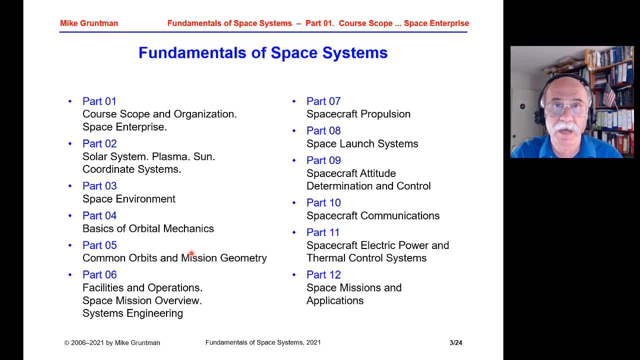 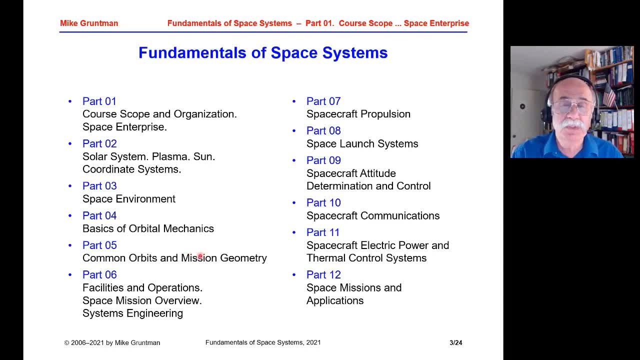 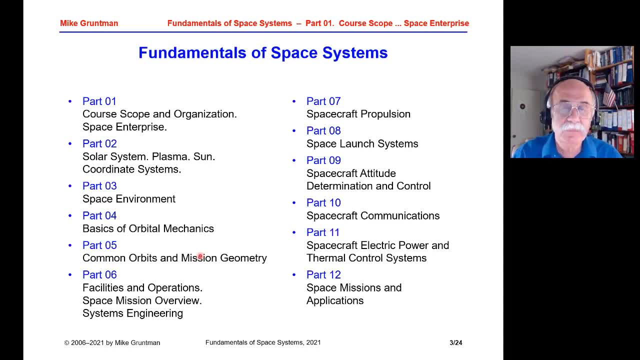 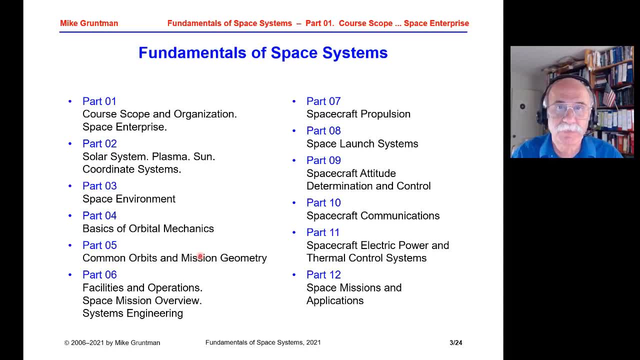 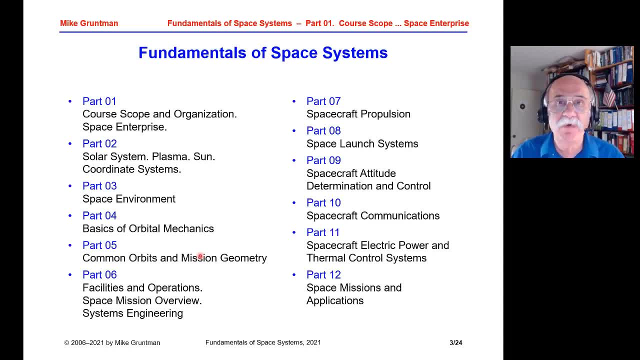 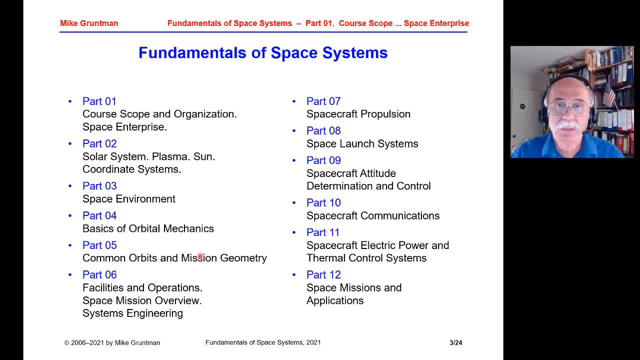 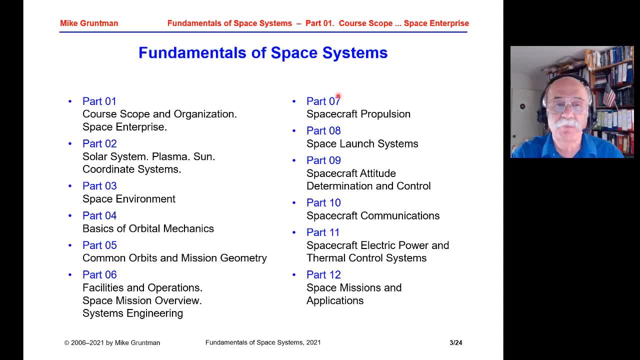 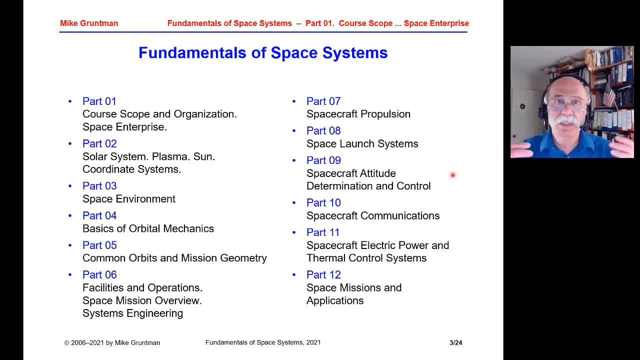 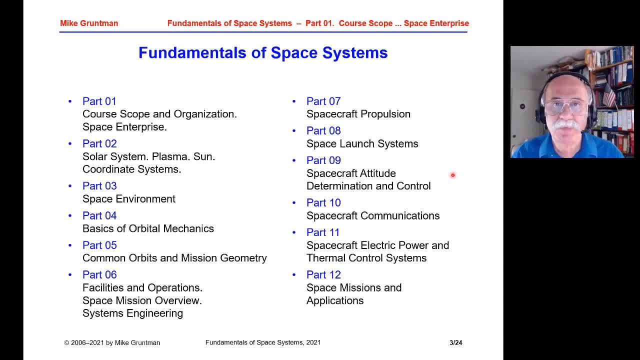 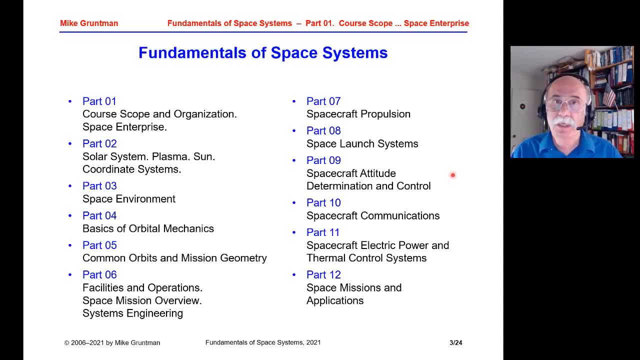 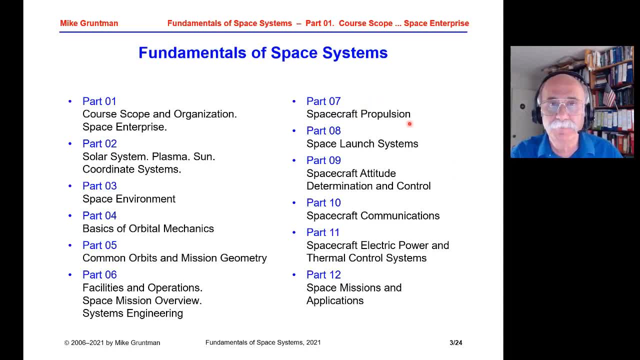 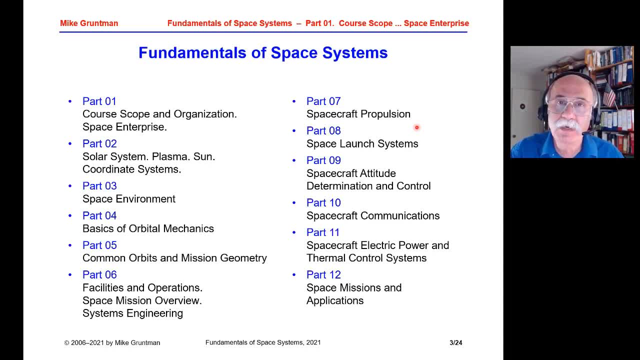 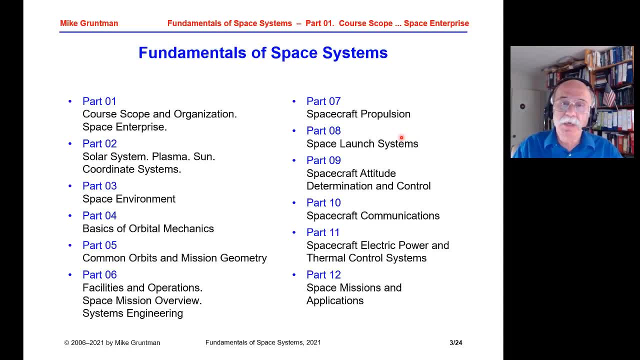 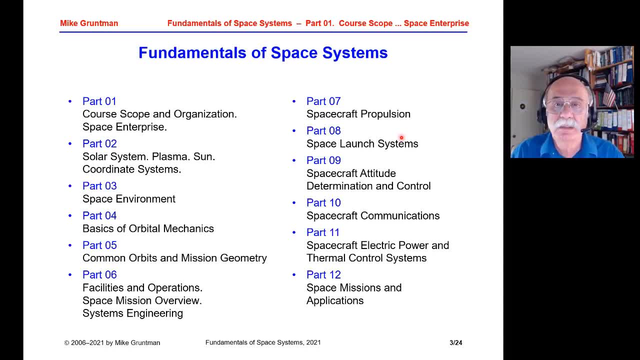 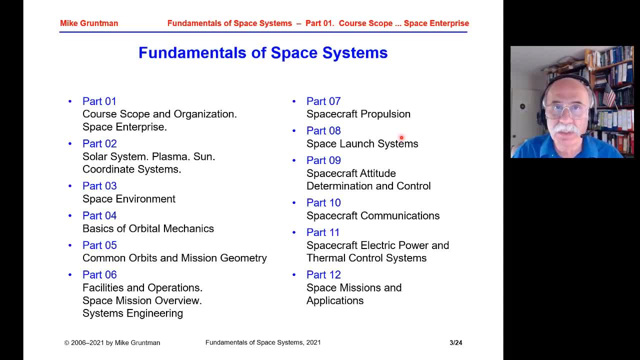 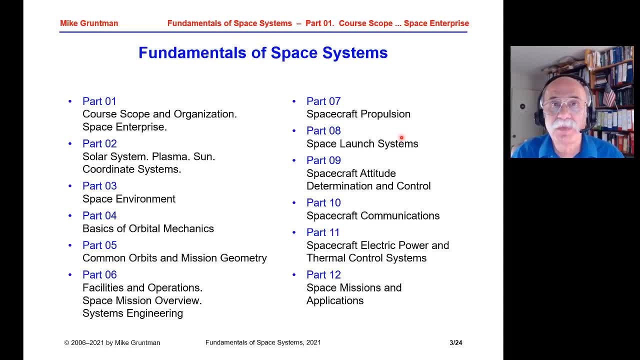 Fundamentals of Space Systems. Fundamentals of Space Systems about communications. it's basically communications between a satellite and a ground station, or it could be communications between the satellites. in part 11 we'll consider another most important satellite subsystem: spacecraft electric power subsystem providing electrical power. 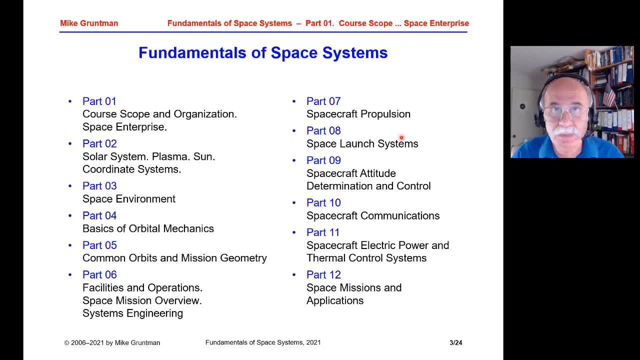 and here there is this, photovoltaic arrays, solar cells, and then there are other possibilities, nuclear systems. and then we'll talk also about the thermal control of satellites, which is just very, very important, because the conditions in space are very different from what we have on earth, on the ground. and finally, in part 12, we will take everything that we discussed in our course. 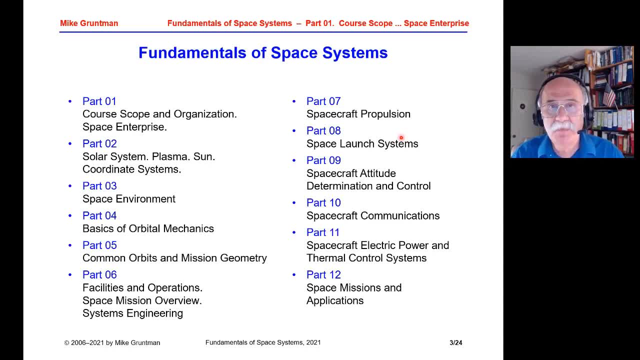 and we will consider space missions in applications in the 21st century, what people do in space, and this discussion would be much more informed because it is based on the previous topics that we considered: the orbital mechanics, environment, attitude, determination, control of satellites, their propulsion, communications, uh power, satellite power. 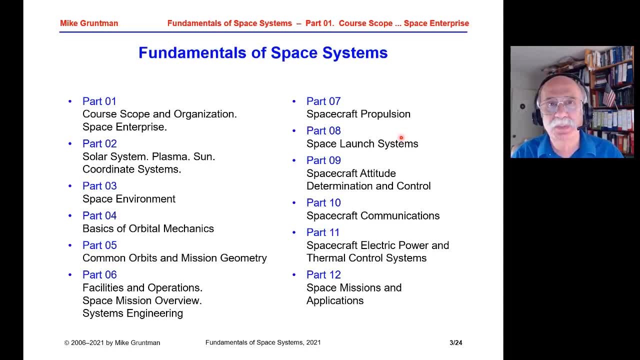 this discussion of the space missions and applications would give us a very good perspective what is being done in space in the 21st century and what is just coming even in the future, and this is in the commercial space, in the science exploration, in national security, in other topics. in summary, uh, this: 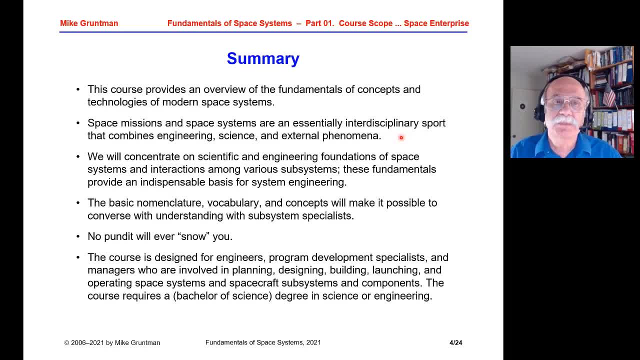 course provides an overview of the fundamentals of concepts and technologies of modern space systems. remember that space mission and space system design are an essentially interdisciplinary. you have various areas of science and engineering combined together. there are also external phenomena, so it's becoming again very diverse areas requires scientific and engineering knowledge. 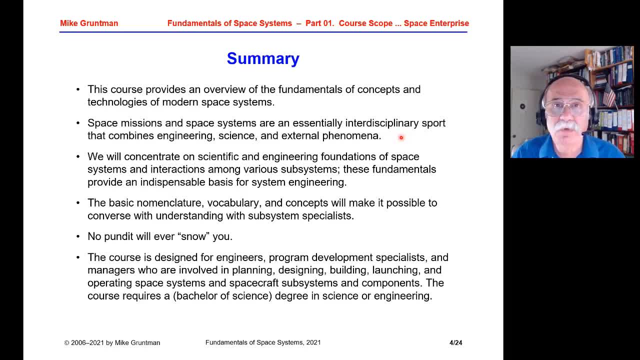 are coming from all possible, in all possible flavors. we will concentrate on scientific and engineering foundations of space systems and how these subsystems interact or affect each other, and the latter immediately brings importance of systems engineering. we will introduce the basic nomenclature, vocabulary and concepts, and this would allow one to discuss with a subsystem specialist. 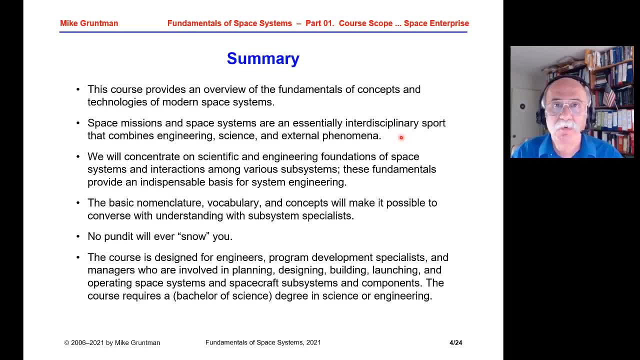 his or her particular area of work. basically, no pundit will ever snow you because again, sometimes you hear it's a very important sounding words and phrases. they are intimidating, but if you know what is behind those concepts, you would understand what's happening there. so this will help you to navigate this with ease. the course is designed for. 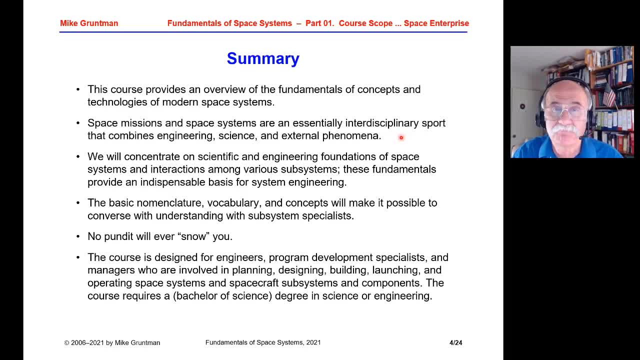 engineers, program development specialists and the managers who involved in planning, designing, building, launching and operating space systems, and particularly for the engineers who are and managers who are coming to space from other areas of work- engineering work, but they are just moving into the space technology. this course familiarizes. 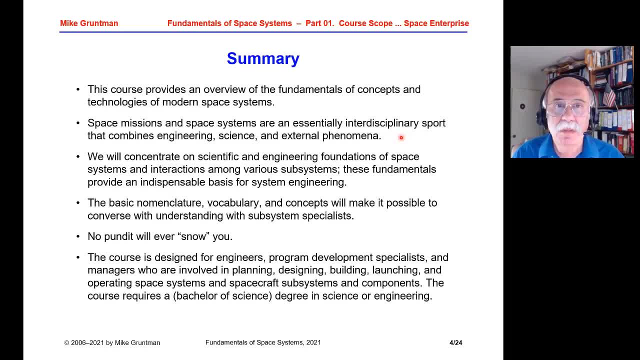 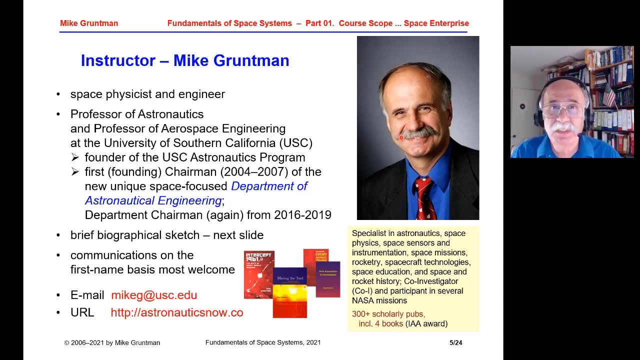 with the global global of technology in space, with the fundamentals of space systems. so a few words about your instructor. I'm Mike Gruntven, I'm a space physicist and I am an engineer. I'm a professor of astronautics at the University of Southern California and I'm also a professor of aerospace and 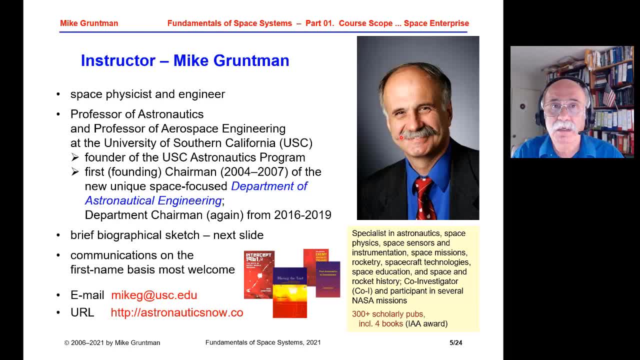 mechanical engineering there. I am the founder of the space program at the USC- my university space engineering program- and I served the founding chairman of the pure space engineering department in 2004-2007. that you see established. typically space engineering is part of aerospace engineering departments and we split from aerospace and we form a 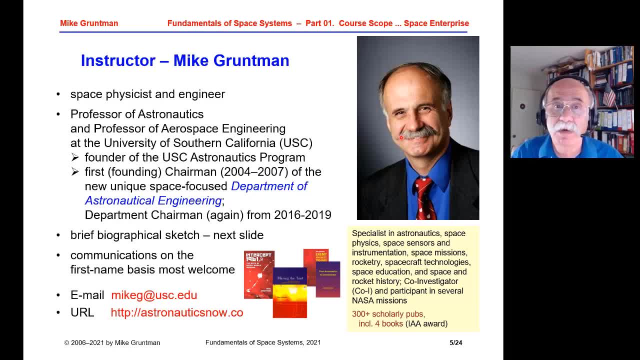 dedicated space engineering department. this is a unique department in the country. I also as a chairman, actually very recently again. the administrative tasks are not very interesting, but we have to do our service. my detailed biographical sketches on the next page. you are free just to look at that in detail if you're. 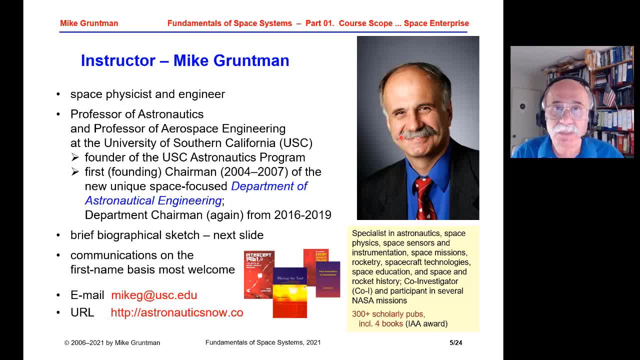 interested, but basically I'm a space physicist and space engineer. I'm a specialist in astronautics, space physics, sensors, instrumentation and other space missions, propulsion, rocketry. I served and I serve now as a co-investigator on the a few NASA missions. I engaged in the research and 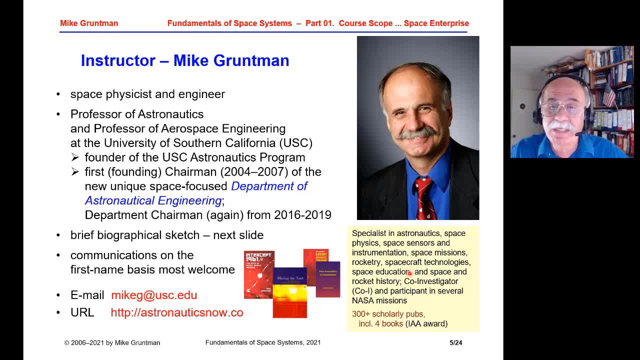 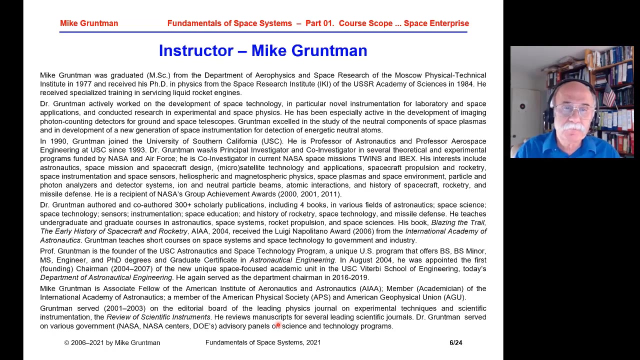 development programs in space technologies, also other government agencies in addition to NASA. I published a large number of scholarly articles, books and all that, so I have a website. it's my website. there should be com letter M is missing here and my email if you ever need to contact me. this is a detailed my biographical sketch, so you. 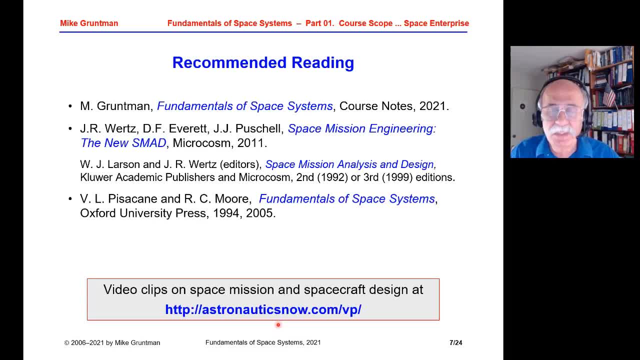 can look at that. what are the recommended materials for this course? well, first of all they will. there are course notes for this particular course, fundamentals of space systems, there on the top. now below, a listed two publications. the first one is the space mission analysis in design, known. 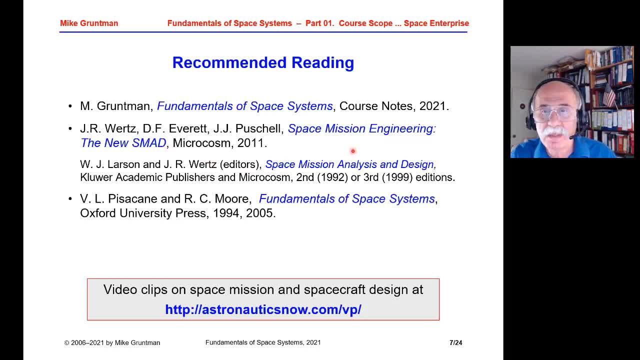 as SMAD. so SMAD was the most widely used book. you could find it on a bookshelf of practically every space engineer working in a space area. this book- the first editions, particularly the second one and the third one in 1990s- became extremely widely used worldwide. every space engineer had it and in 2011, 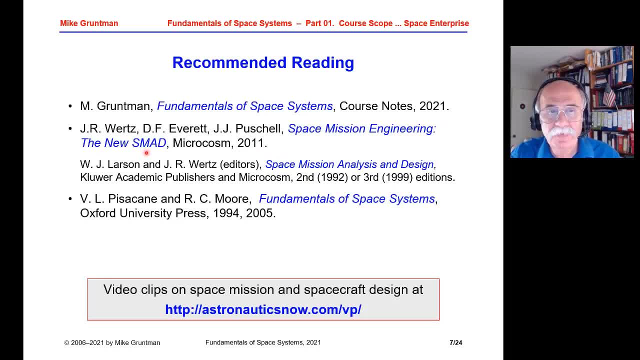 the new edition was published the same authors or editors, because these books are compilation of contributions by specialists in the field. the new edition- the new SMED as it is known, will become one has become the replacement for SMED. again, it's very widely used. but if you have the old version, please, 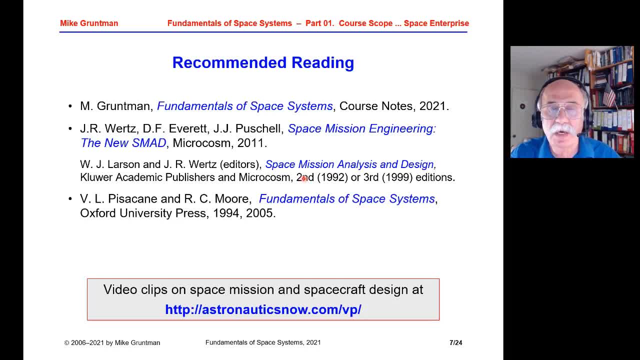 do not dispose that. keep it because while the new SMED repeated a number of fundamental foundational topics in space engineering, it also added the new topics and because the volume of the book grew dramatically of the new SMED, it's really a big, heavy brick. because of that some topics from the old edition were discarded. 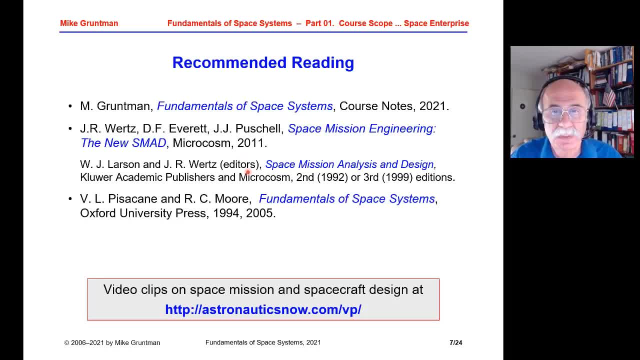 but they still are foundational. so both of these editions are very important. and there's also another publication just coming from a different group of authors: fundamentals of space systems. that is more sort of a science orient on the fundamentals of satellite subsystems. in addition to these two, 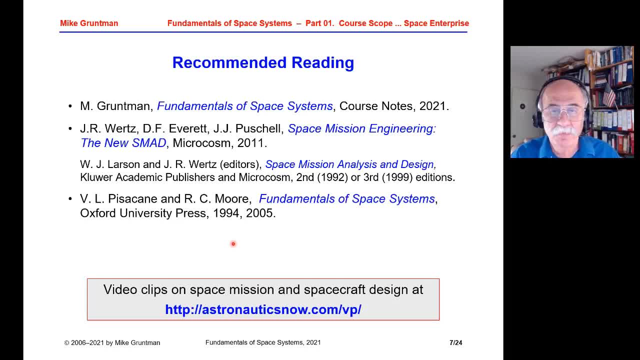 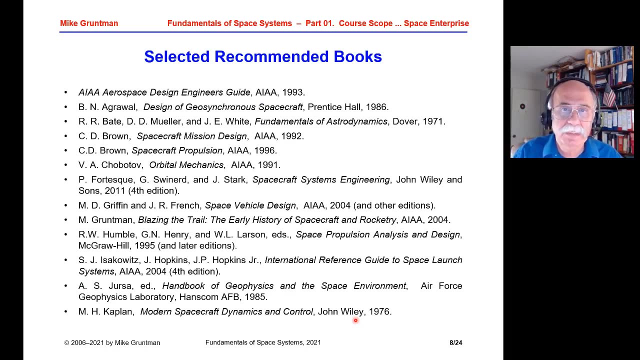 bad books. there are very large number of publications. at the bottom there is a website- this is the website that I maintain- that lists a large number of publications there. these next two slides, two dozens of books in various areas of satellite technology and listed here and again at the bottom there is a website. 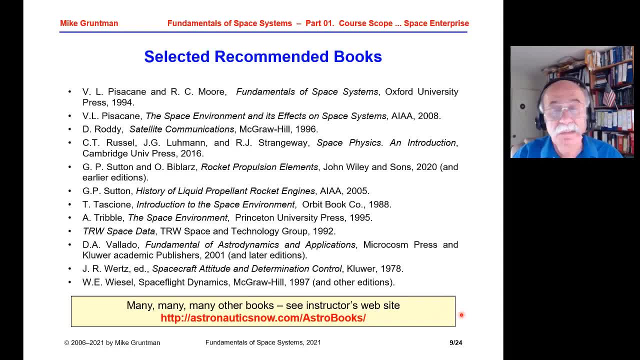 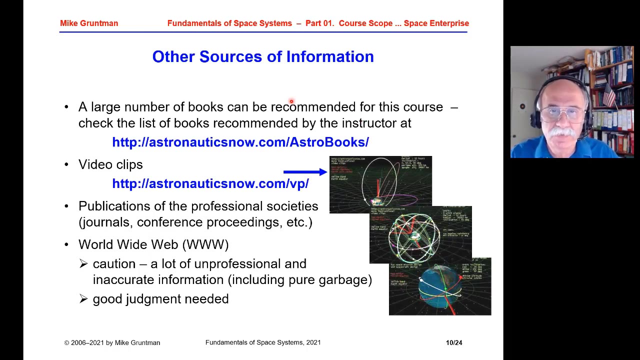 that lists ten times more titles of books and they they are compartmented in the different areas: attitude, determination and control, spacecraft dynamics, orbital mechanics, propulsion and so on, so forth. what are other sources of information? so we already talked about the books on my website I have. this is the URL. I have about one dozen short video clips. 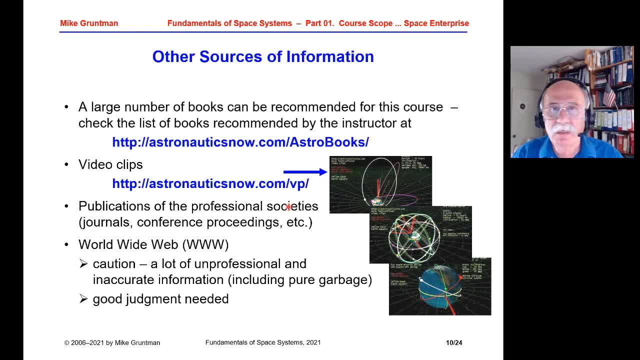 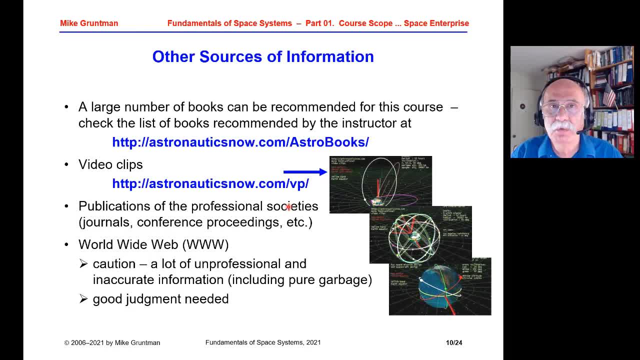 or illustrate evolution of space spacecraft orbits. now, if you your background is not in orbital mechanics- a lot of concepts talking about regression of nodes or rotation of the line of CDs and other very important concept that describe what's happening with the orbits of satellites, and we will be talking more. 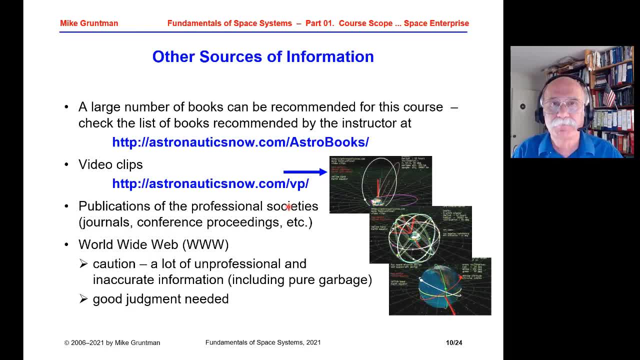 about that in the orbital mechanics part of this course. so but a lot of these concepts is a very hard to visualize if you are not from this particular engineering area. these videos that just demonstrate evolution of orbits, I can tell you that watching how the orbit evolves in time is not very exciting. 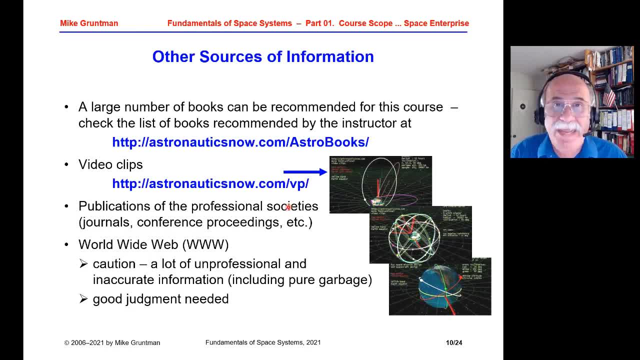 it's boring, like watching the paint drying, but it's very important. provides a very good visualization what is happening with when you put satellites in orbits and satellites never stay in an orbit where you put it because there is some disturbing forces as well. administrate some forces. 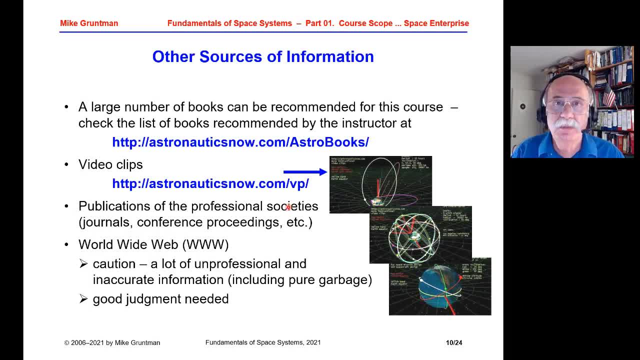 will discuss during the in this course. later that will start changing the orbital properties of satellite. so it's again. it's about a one dozen. one dozen video clips there, five minutes long. they're all on YouTube so you can watch them and pull them out. pull them out and study in the detail, if needed, then there. 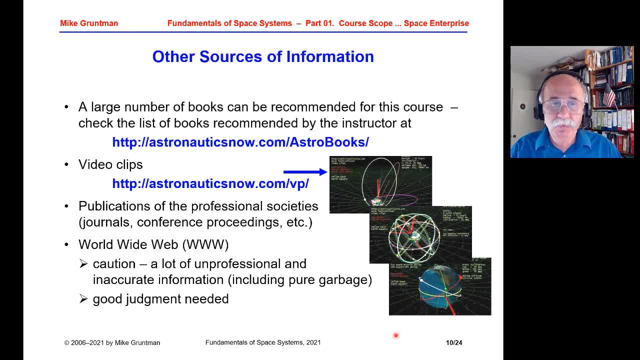 are obviously publications of professional societies. in addition to books, it's journals, conference proceedings, textbooks. they're very important and there are a lot of information on the World Wide Web. here one have to be careful, as with almost everything on the World Wide Web, because we have some very useful and solid information there, especially a number of. 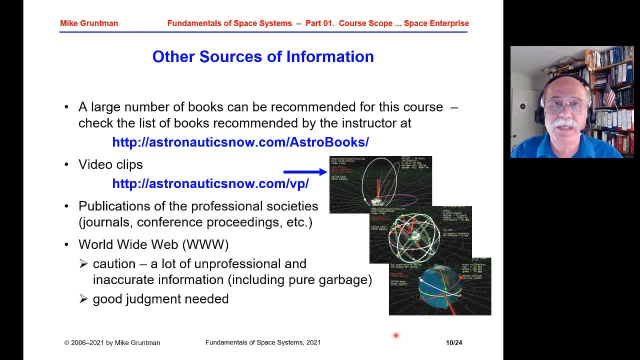 PDF files of government reports, technical manuals or technical publications are there, and then there is nobody really controls that what's going up there. so there there are a number of postings of basically garbage. it's a lot of inaccurate information, so you have to be careful, and this is like with everything else on the web: a lot of. 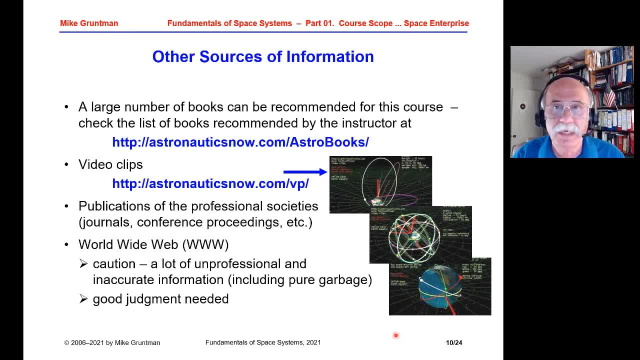 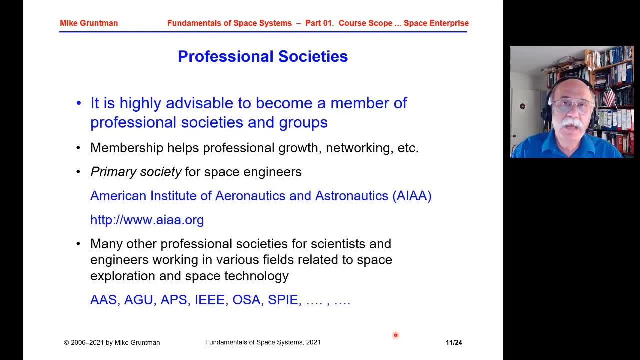 fake, fake stuff, fake news and basically uninformed things are there, but a lot of very, very good things. so it's a judgment is needed. professional societies play a very important role in space technologies, in any other area of science and engineering, so it's a very important if you are getting into the. 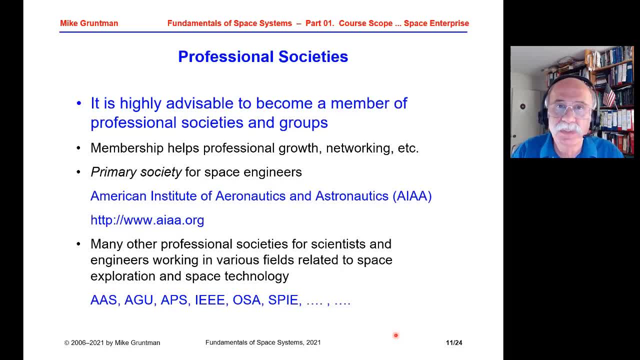 space area to become a member of technical society. it provides networking, opens a very important connections and the then the publications- technical publications- of the society's and conferences and the meetings, forum, forums are very, very important in space engineering. the primary societies, the American Institute of Aeronautics and 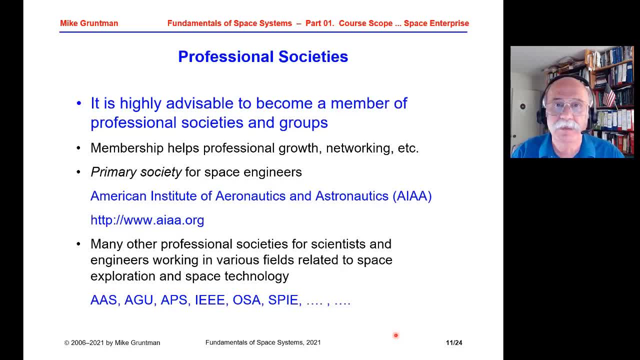 Astronautics, AIAA. this on the this course is part of one of the AIAA's courses, and but there are a number of other societies that engaged in various aspects of space technology, and just I listed just a few: American Astronautical Society, American geophysical Union, American Physical Society, IEEE, OSAS, PAE. 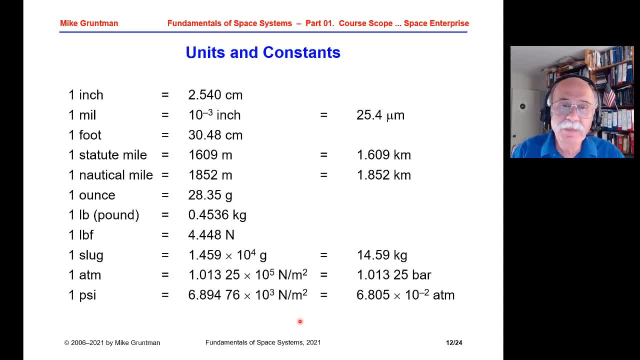 and many, many others, and finally, in this first half of this lecture and note on the units and constants. the aerospace field is famous or notorious, depending on your perspective- on using all kinds of units. there are metric units, there Imperial units, there are other non system units and the situation is not going to change, regardless whatever regulators or just. 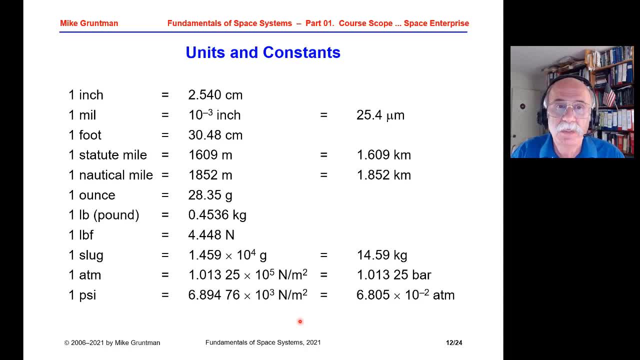 governments may tell us to do or what not to do. because of that, it's very important to be very, very confident in juggling with the units. to be confident in using different units. it does mean that you have to be able to say, do estimates or solve problems in different. 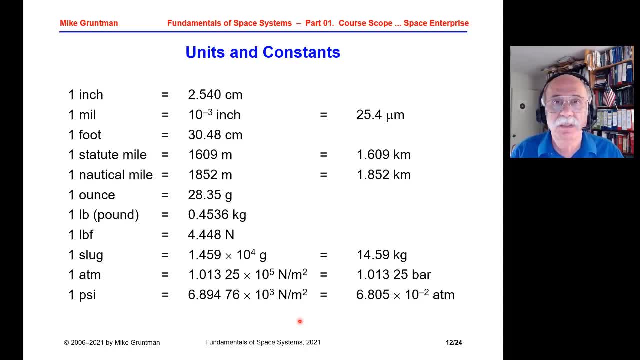 systems of units. you do it in your preferred systems, just in the metric system, for example, but you take the parameters that are given in other system of units, convert to your preferred system. do you do your calculations or consider what's happening, do your design and then when? 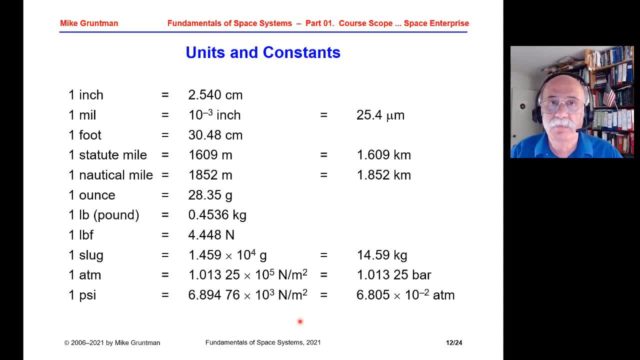 you get the results, you convert them to the system of units designed by your customer. because you cannot tell to a customer that well, you don't know the units, so you just cannot do the job. you will lose that particular customer. then if you units and constants listed here so will help for you in this course. it's. 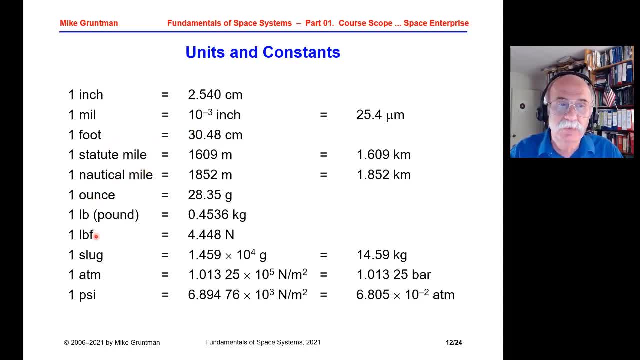 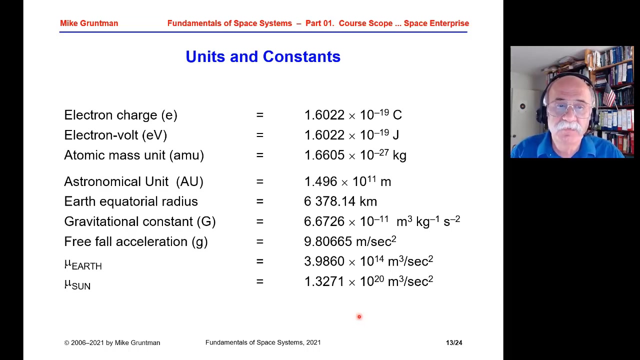 inches mills, thousands of an inch, important units, and I will be talking during the course. you will see them. but in again in the technical literature, particularly in the United States, you will see this: a combination of various units. this is like this page. this slide is for for reference. the next slide is a compilation of a few important physical 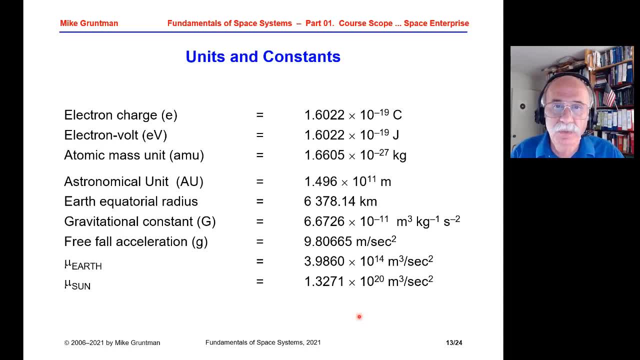 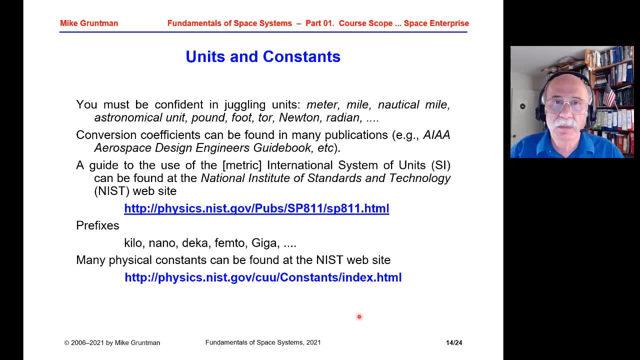 constants that are being used and I also want to provide you to URLs, to links to the resources on the web. the National Institute of Standards and Technology, the former Bureau of Standards and Technology in Chicago, has a website where there is in the document, so I am giving this URL here and on this website they're changing URLs. 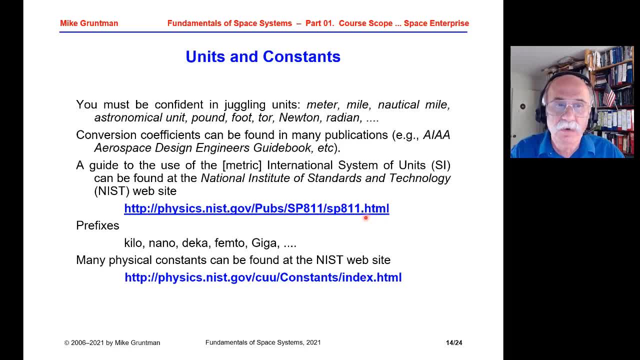 as a PDF. this document is a guide to the use of metric SI international system of units. although it's a guide to use the metric units, it includes multiple different units, all of which. I just have to imagine how they are organized. it's five meetings. 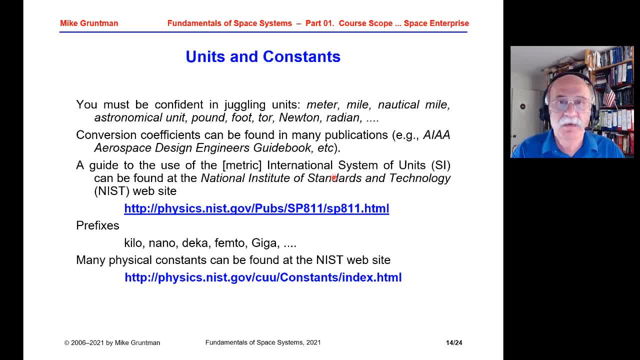 it has a very extensive list of conversion from non-metric units to metric units. so it's basically: you pull out this document, you print it. i think it's 50 or 100 pages. you print it, you one time put it on your bookshelf and it will stay for you for the decades. it will be a very, very helpful. 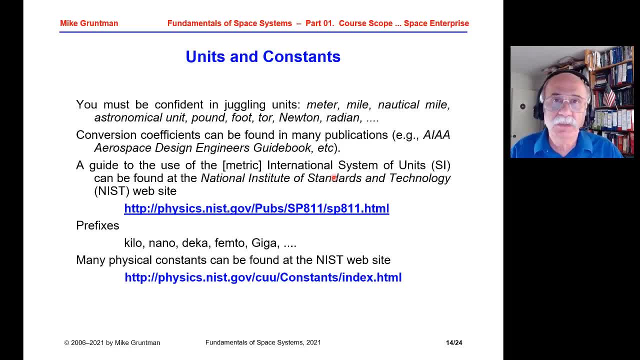 resource. the national institute of standards and technology is also the main repository of the physical constants constants and all that. so they have also a website from where you can download the latest definitions of main physical constants. although the physical constants really do not change much of, and if they slightly adjusted it very unlikely would affect your 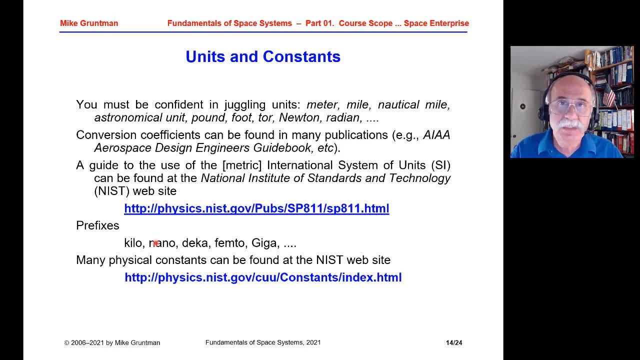 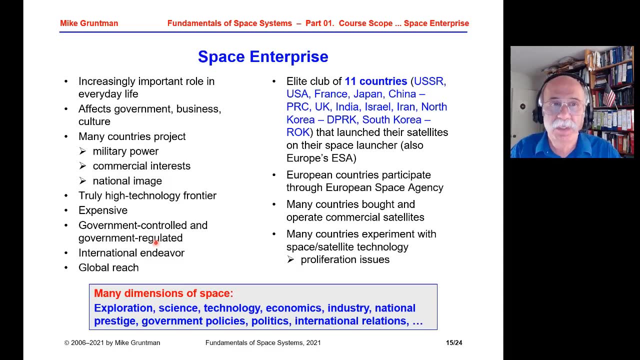 applications, but still this is a very nice compilation from the ultimate authority in the country on the constant. so these two documents just would be very important to download and just keep them on the bookshelf. now let us switch the gears and talk about space enterprise, space plays. 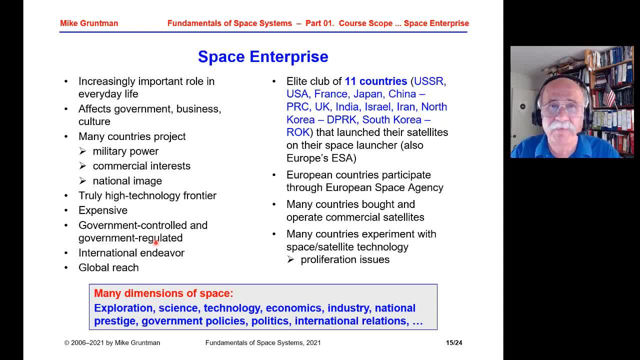 an important role in the everyday life and its role actually increases all the time. it affects government, business, culture. many countries project military power, commercial interest, image prestige. it's also truly technological, trans frontier, it's expensive and it is also government controlled or government regulated. immediately tells us that the 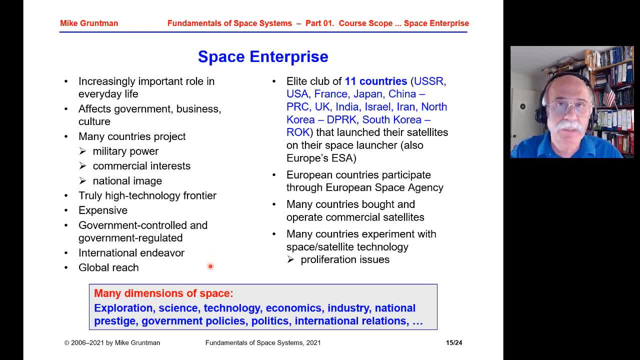 role of national policies, and sometimes even politics, becomes very, become very important, and it's also international in its nature. there is the elite club of 11 countries that built their own satellites and launched them into space on their own space launchers. it started with the soviet 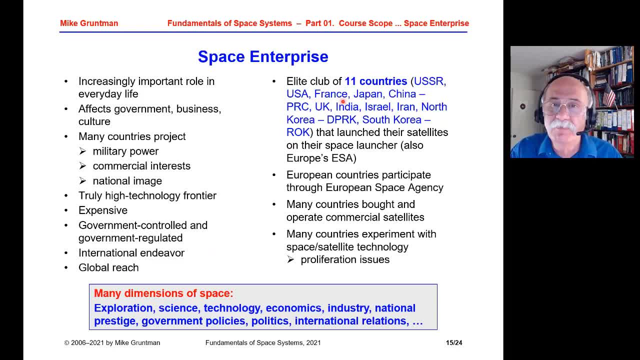 union and then the united states. then it was followed by france, japan, the people's republic of china, united kingdom. after that there was national space launch programs in europe. stopped europe, western europe, combined its resources in the european space agency and the european space agency would later start is isa would start launching its own satellites. 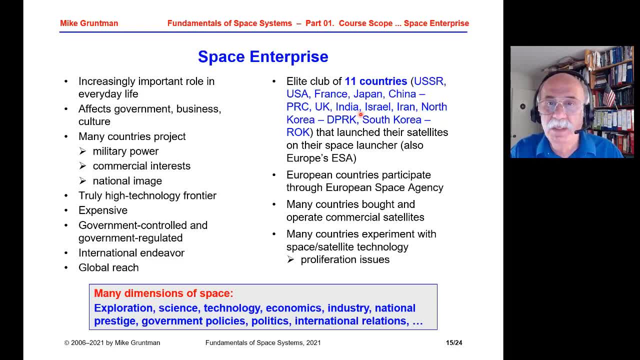 on its own rocket launchers. then india launched its own satellite, israel, iran, north korea and then the south korea. european countries, as we mentioned, participate through the european space agency issa. in addition to this elite club, many, many countries bought and operate commercial satellites. they are launched by countries that they're capable of launching. 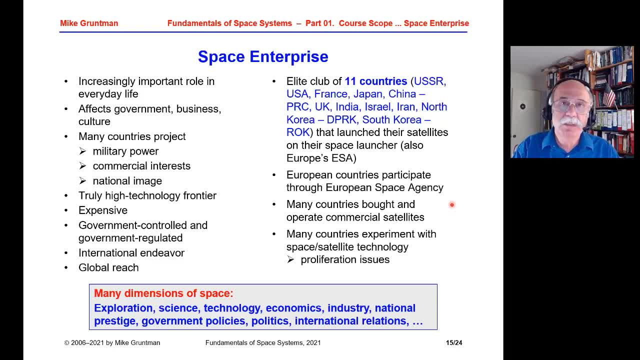 satellite satellites, so that the number of countries that bought satellites or even started to build their own, but they are launched by other countries for them, is growing dramatically. many countries experiments with space technologies, So this brings an issue of proliferation of the technology, because in science and engineering really there is no such a thing as a civilian science or civilian technology. All science, knowledge and all technology are dual use. 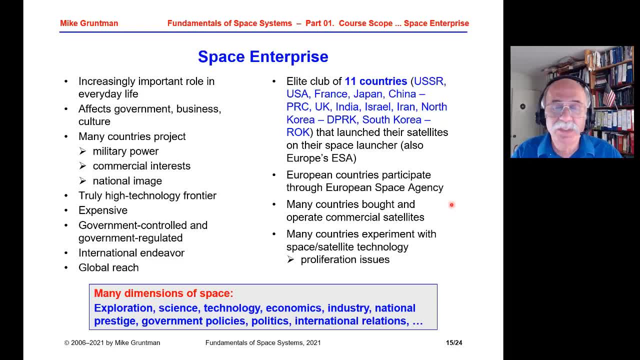 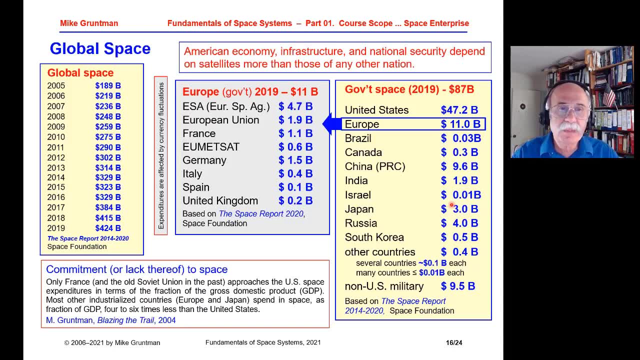 There are many dimensions of space exploration: science, technology, economics, industry and national prestige, international relations and so on and so forth. If I look at the global space in economic terms, on the left, you see that the globally space enterprise is growing and today it's more than $400 billion per year. 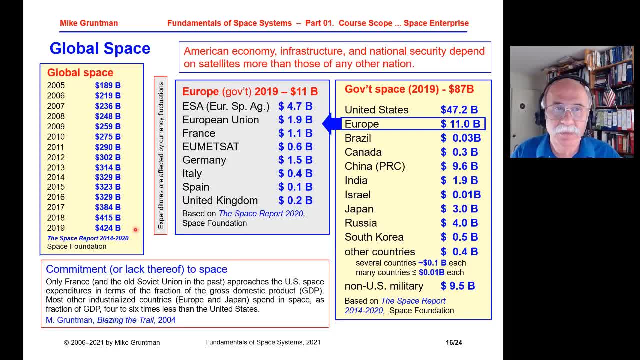 These numbers that are given here. they are applicable, They are approximate, and one of the reasons is that the way how they are calculated evolves with time and then the currencies fluctuate. but it shows you the significant growth. for the last 15 years it's roughly 6, 7, 8% per year. There was a growth of the international space enterprise. The American economy, infrastructure and national security depend on satellites more than those of any other nation Until mid-1990s. in dollars annually, Governments in the world spend less than one quarter, close to $90 billion. 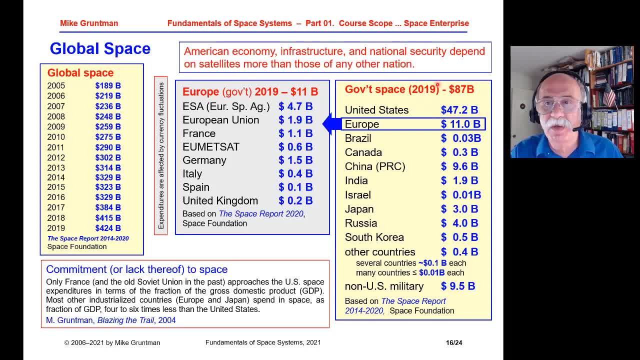 The United States government spends one half or even more than one half. what other governments spend globally, With the exception of trade and economy, Whether any other economy or any再 κ forgiven doesn't stop. Part-time income is honestlyoffering a switch between government and international millones only. 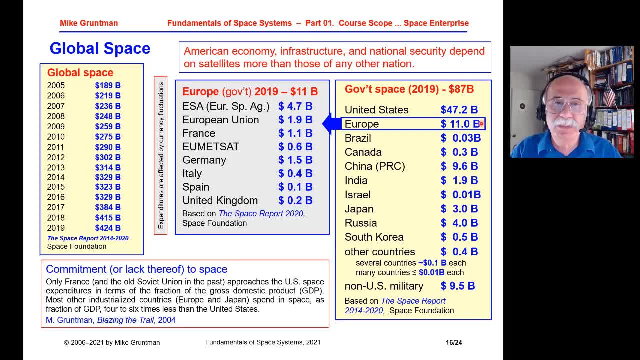 globally on space. in the United States government is very active in space and in the second you would see the numbers from a different perspective. Europe is combined. Europe is four times smaller than the United States and there is the breakdown of the main countries that spend the money in space. it's good. 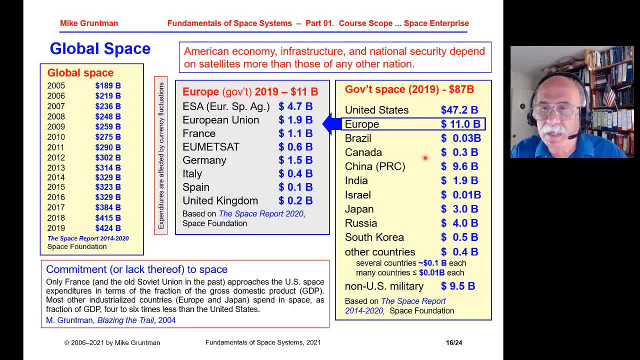 governments. in addition to Europe, there's: Canada has a space program, obviously. the Soviet Union or Russia today has a major program. the People's Republic of China has a rapidly growing program. India, Japan, has a healthy program in many, other, many other countries. then there is also non-us. 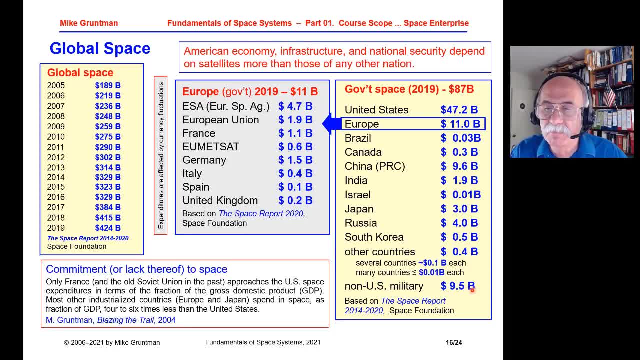 military space total combines about ten billion dollars in the moment. and then there is the United States, and the United States government will talk about the United States military expenditures in space. in 2004 I made a statement and I got actually a lot of flack from some European friends. 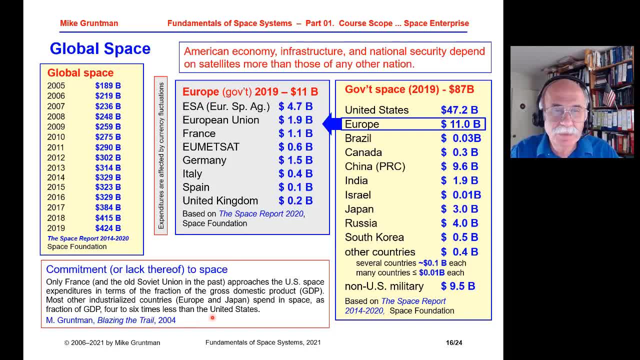 unfortunately especially- and I just basically wrote that only France and the old Soviet Union in the past approaches the United States space expenditures in terms of the fraction of the gross domestic product. other countries spend like four to five times less governments that the United States government table on the left. 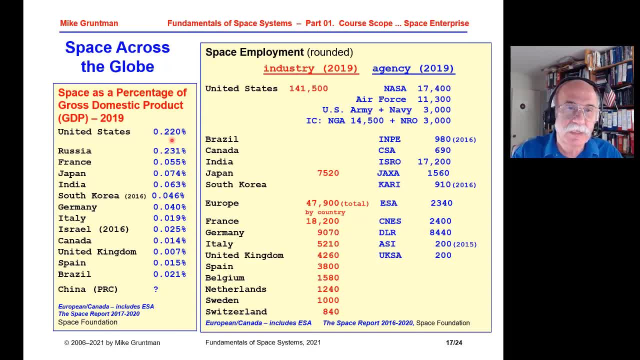 demonstrates that. so you see, this is the expenditures of the United States and all European countries in Japan they spent. if you look here carefully, at this table, at your, when you have time, you will see that they are spending really four and five times less than the United States. this is basically nothing. 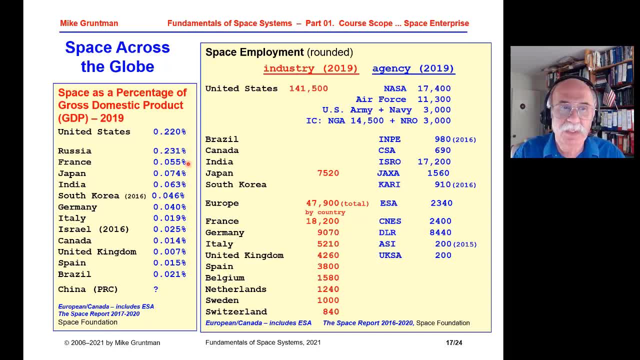 change in terms of this ratio during the last 15 years. Russia and the summit union on the past spend the best, spends about the same as the United States. is a fraction of GDP, the gross domestic product. we don't know too much about China because it's a communist country. there's economy, or? 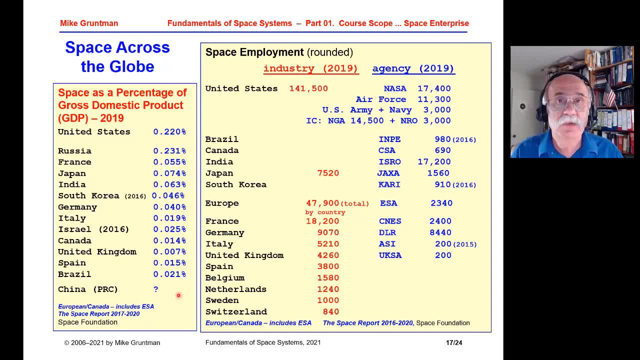 accounting is not transparent, so you hard to say, but you can be assured that China's fans probably even more than the United States as a fraction of the gross gross domestic product. but it's important that again, in terms of government spending spending, European countries and Japan spend significantly less And so they are basically not committed to the space exploration and space technology to the same degree as the United States government. 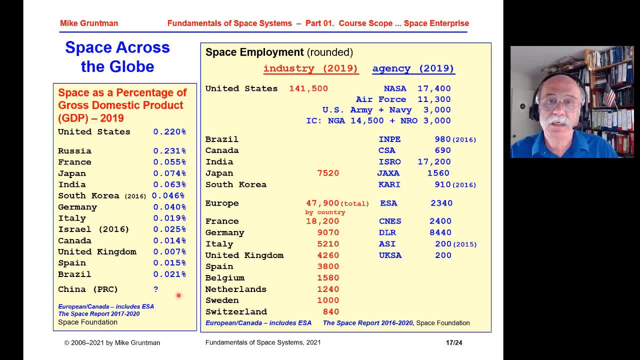 Now, if you look at the space employment in industry- in the red, and in the government agencies, in blue also, the United States dominates with these numbers. We don't have numbers for China or for Russia to that matter, really, But you can see that the United States, commercially, it's almost 150,000 and Europe total just three times, three times less, And there's a breakdown in the space employment. 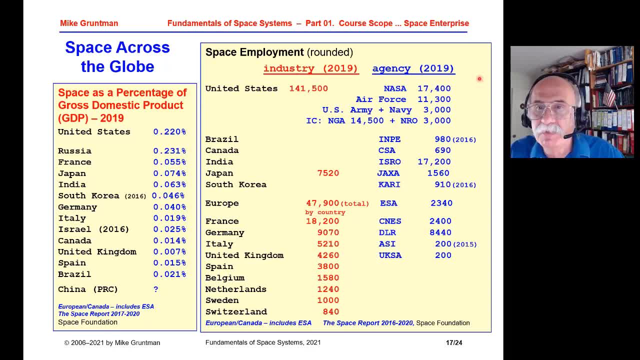 And in terms of in the, according to the countries. if you look at the government deployment, NASA is about 70,000.. And then there's a military, approximately the same number of employees and other government agencies in other countries. I know that the India has a very large number of the employee, government employees working in space. 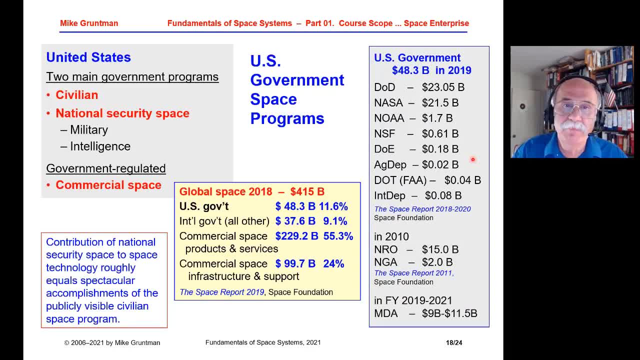 Look at this table at the time convenient for you. Let me just talk a little bit about United States government space programs and there's an also there's an illustration here that the numbers that we have they're approximate, and it's because it's not clear how to tabulate them. 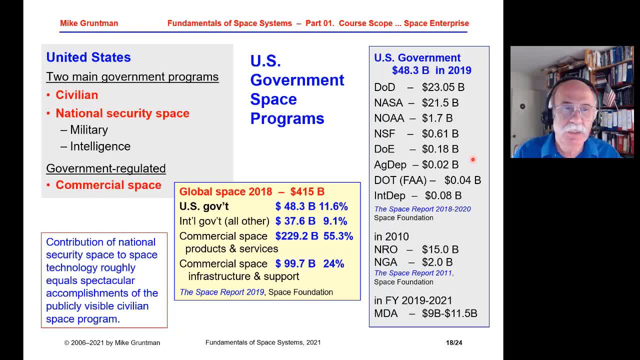 The first of all. traditionally people talk about that while in the United States there are two government programs, civilian and military. Well, in reality there are three government programs. They occasionally talk to each other, They occasionally cooperate with each other and sometimes they don't talk to each other and operate independently. and their size and not very much different from each other. 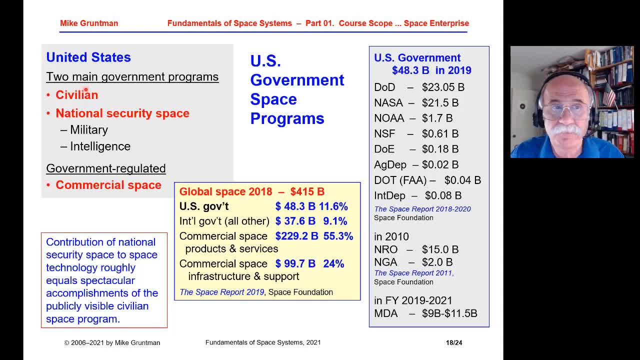 These are the civilian program. This is primarily NASA, And then there is a military, which is a department of defense, And then there is the intelligence community is basically space reconnaissance. So in the national security space There is a military. These two programs. 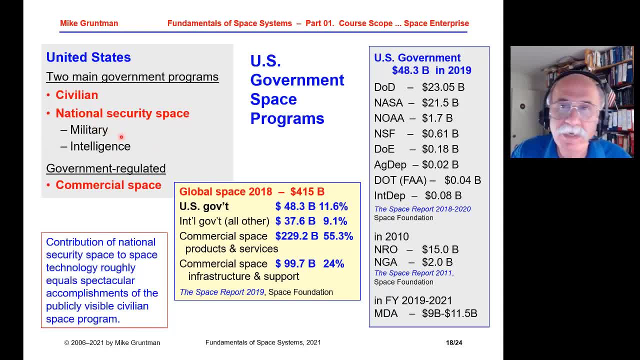 They're not very much different in scope and in the contributions, But when people talk about the military space they usually do not distinguish them. But again, these are the two programs with the two stovepipes of the people would say in government. These are the two programs that occasionally talk to each other and sometimes they don't talk to each other. 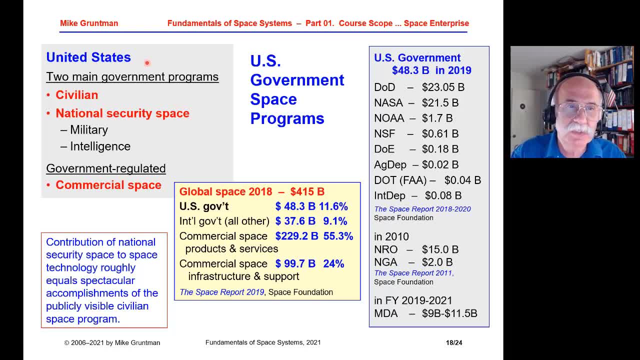 And in addition to these three main government programs, Okay, We have a commercial space that is very heavily government regulated for these reasons: It's national security and safety. If we look at some numbers on the right of the government, so these are from the Space Foundation, just the current numbers saying United States government $48 billion. but this is without intelligence program, without that one. 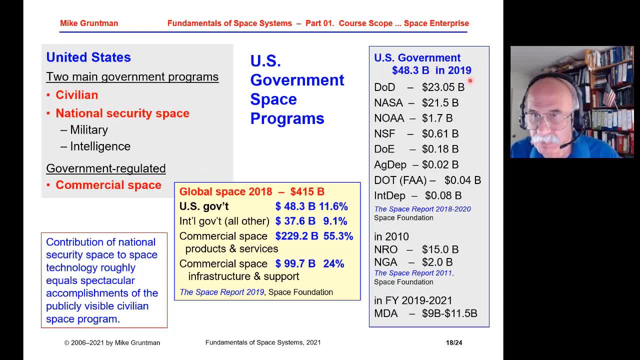 And the breakdown. so it's about half of this government spending shown on the right is Department of Defense, it's military space, And then there is a NASA and just a little bit sprinkles across other departments in the federal government. How much goes to the intelligence space Reconnaissance is a classified number, but for a couple of years it was not classified. So in 2010,, for example, National Reconnaissance Office and National General Assembly. 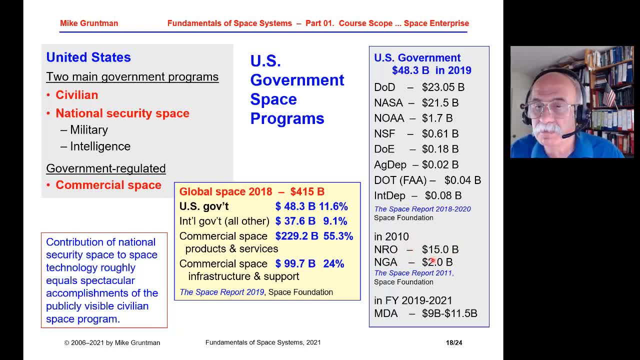 And there is a whole bunch of geospatial intelligence agencies that were close to $17 billion in 2010.. Just tells you that this is about the same as the Department of Defense spends Basically. you can think about the United States government programs: three programs roughly the same size: Department of Defense, Reconnaissance and NASA civilian space. 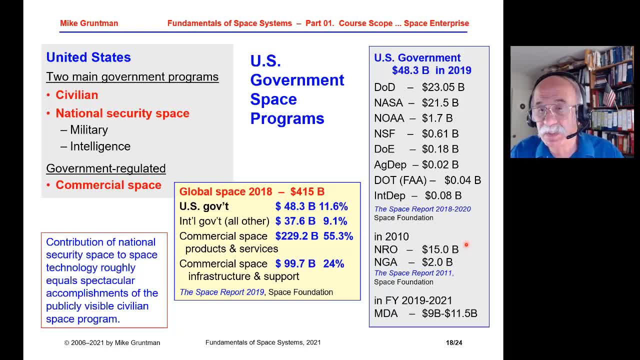 In addition, there is a missile defense agency. that spending between NASA and the US is about the same, So this is about the same as the Department of Defense spends nine and eleven billion dollars each year, and they relies very heavily on the technologies, either space technology or close relations to space technologies. 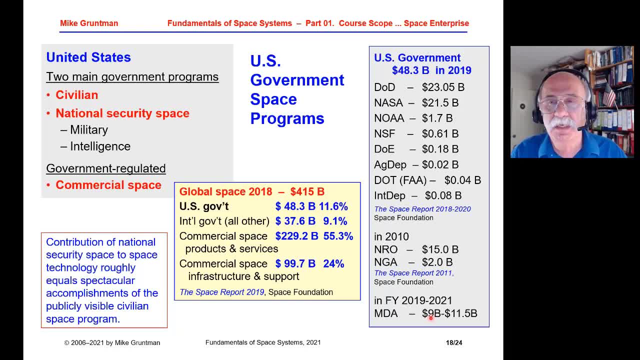 and these kind of expenditures. it's again, they're linked to space if you look in there from the engineering point of view, the same contractors that are working in the military space, intelligence, community space and the NASA, the same industrial contractors engaged in the missile defense work. this 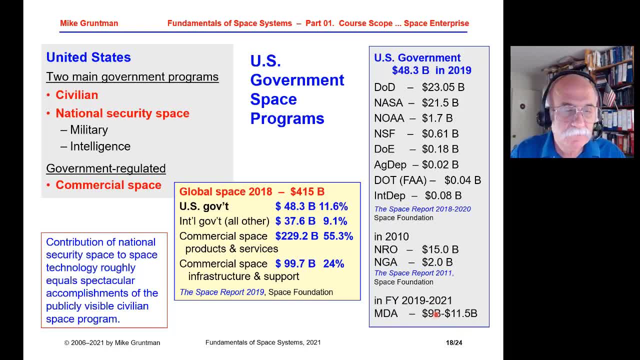 could be considered as the part at least of them, of the space engineering, and we'll talk about a little bit more about that in our last lecture, lecture 12, when we will discuss what is being done in the 21st century. otherwise, if we forget about again this missing intelligence contribution, 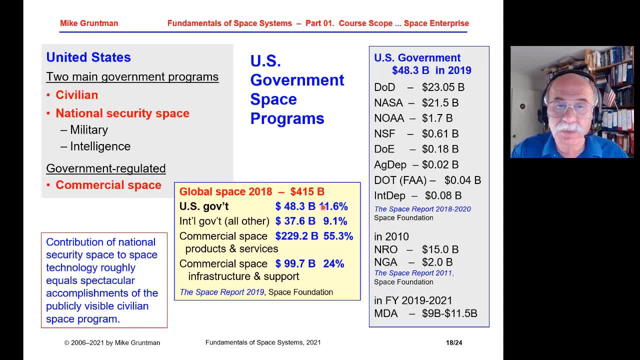 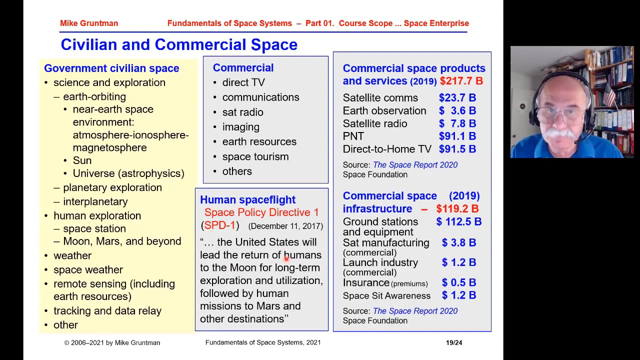 so the United States government- 48 billion dollars, which is 11% of the total global space commercial and government. across the world, commercial space dominates 55%. and then there is a commercial space infrastructure. we'll talk in a second about that. it's one quarter of the total expenditures. what? 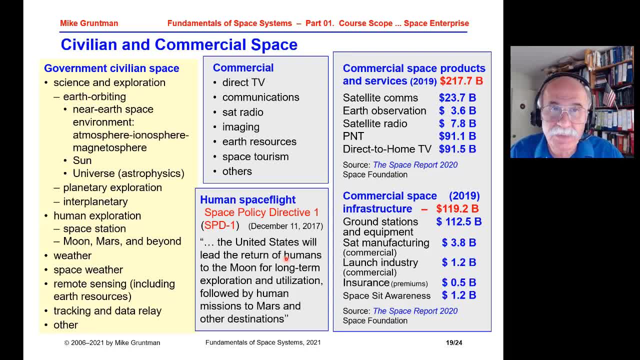 is being done in the government, civilian space and the commercial space. first of all, on the left, government civilian space, it's a science and exploration, and here there are two main thrusts. first, we explore the solar system, the Sun, the universe, from the point of advancing scientific knowledge. 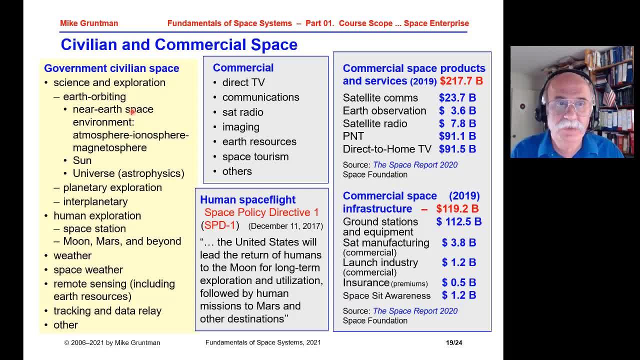 we want to learn about the nature. the second thrust is our spacecraft operating space environment and we want to know how the magnetospheres, the Sun's activities and everything else affects our space system. so there is this applied component. this is the government, civilian space. the focus focused on these. 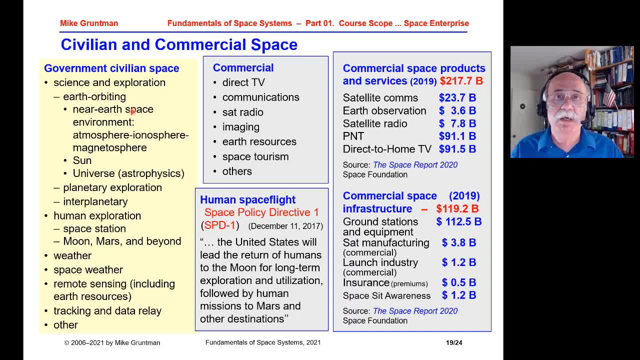 two thrusts: to learn about nature and apply our understanding to understanding of the environment: space environment and interactions from the space systems. and There are Earth-orbiting satellites doing that. They study near-Earth environment, atmosphere, ionosphere, magnetosphere. They study the Sun. Then there are satellites that go to other planets in the interplanetary space and then do planetary exploration. 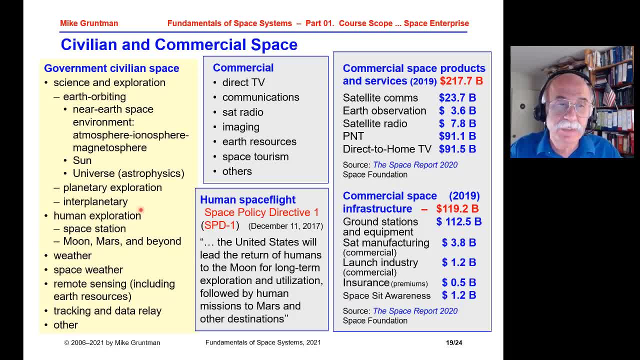 Then they will have a very large program in the human exploration. It's the International Space Station- Again in section 12, last section of this course, we'll talk more about that- And they're going to Moon, Mars and beyond. 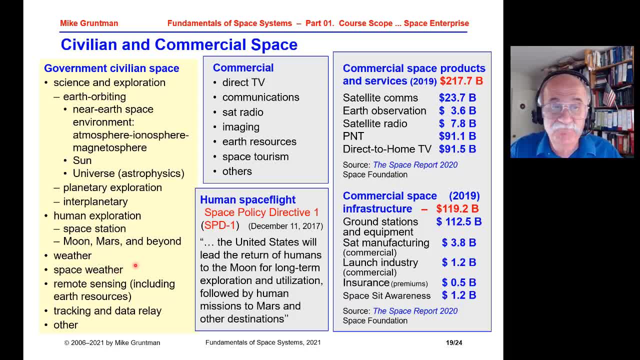 There are government satellites doing weather, space weather, remote sensing and many other things. In terms of the human spaceflight, there was a major decision made in 2017.. The spaceflight was made in 2017.. So-called Space Policy Directive 1, that the United States will lead the return of humans to the Moon for long-term exploration and then will go to Mars and beyond. 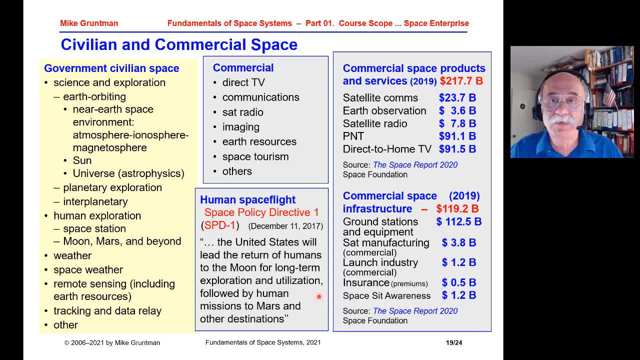 We'll talk in section 12 of the course. In terms of commercial, a lot of things are being done: Direct TV communications, satellite radios- Now you buy a car and it has a Sirius XM satellite radio there- Imaging stations, Radio of the Earth resources, Space tourism is coming and many other things. 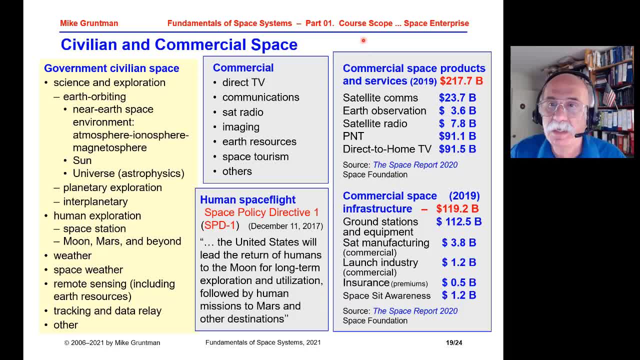 In terms of numbers of expenditures. on the right, we have some numbers: The commercial space products: $220 billion internationally. What is the leading industry in space? This is direct-to-home TV: close to $100 billion. Look at the space satellite communications. 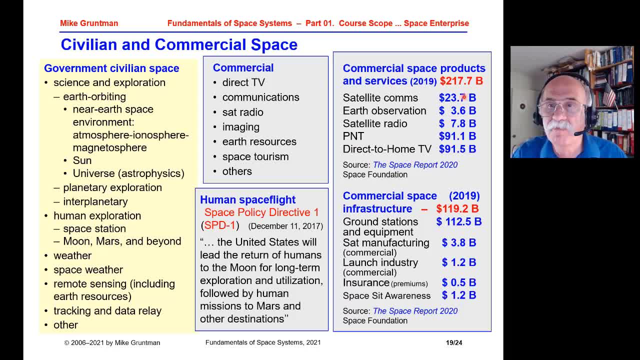 Communications through the satellite. It's four times smaller. Earth observation, remote sensing, significantly smaller. Satellite radio- now $8 billion, again also smaller, So it's direct-to-home TV dominates. Another huge area is PNT: positioning, navigation and timing. 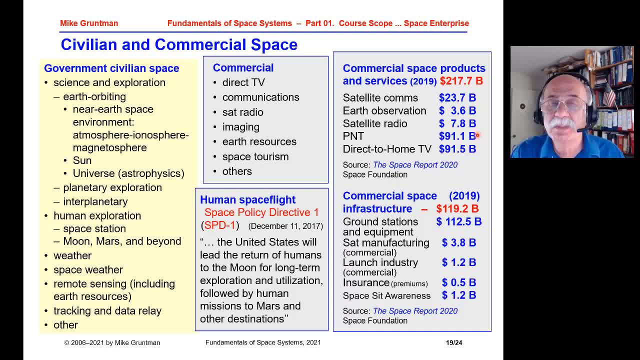 We'll be talking more in the course later about that. This is basically GPS, the global GPS. This is basically GPS, the global GPS. This is basically GPS, the global GPS. It has a global positioning system and it's analogues developed by other countries. 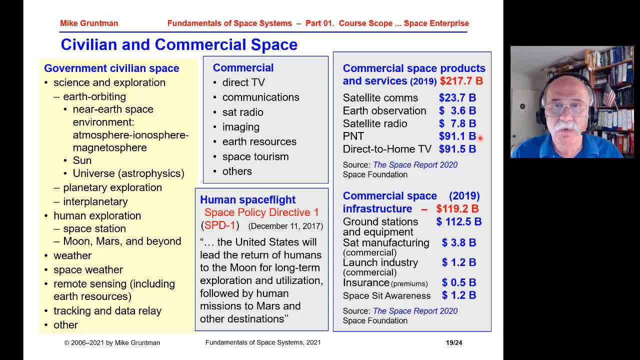 And we know that GPS is ubiquitous, just in almost everywhere we have it. And then there's the commercial space infrastructure, which is primarily ground stations and equipment that is supporting our satellites, getting data from satellites, communicating with them, and so on, so forth. 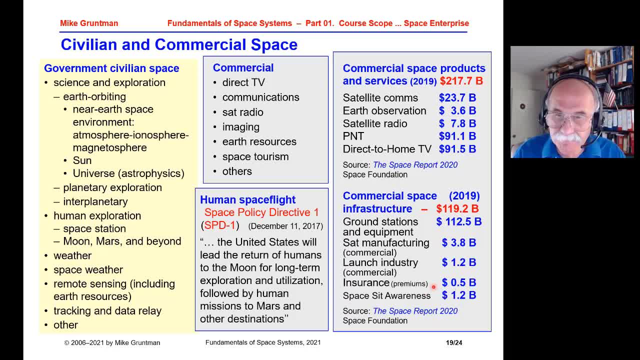 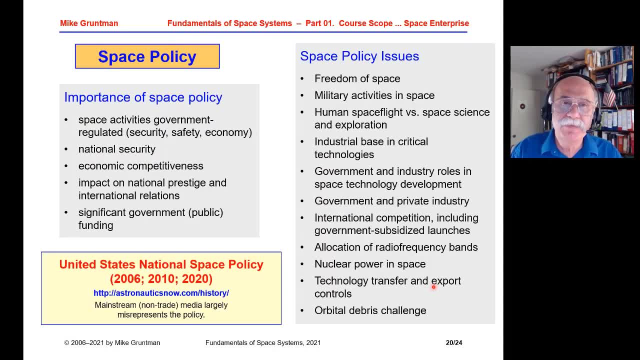 And then there's some other mining systems And there's some other mining systems And there's some other mining systems- minor, minor activities, because what happens in space is either government controlled or government regulated. because of that, space policies, national space policies and politics because of that, become very 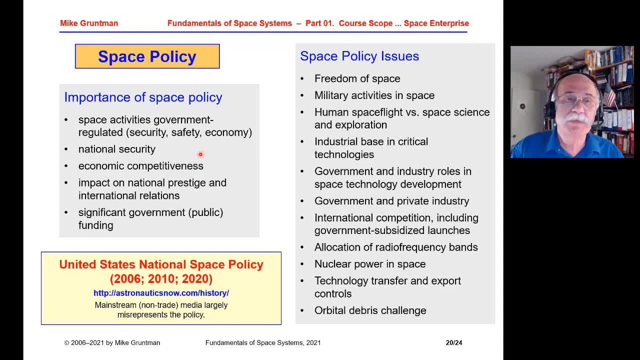 become very, very important. government regulate space because of the security, safety and the economy and the expert control and other things. national security involved the economic competitiveness involved, its national prestige also and a lot of again in the government control space. it's a lot of public funding goes there. now the united states publishes. 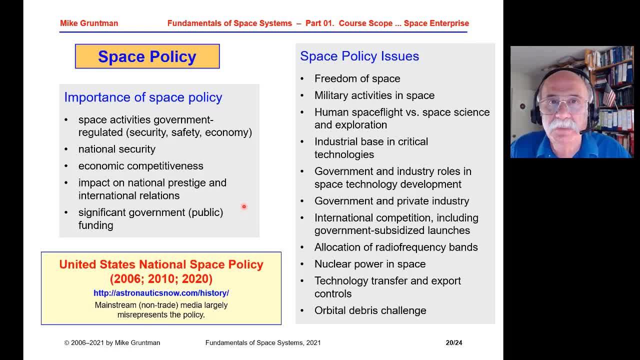 national space policy. basically every presidential administration issues its space policy. i have on the web- actually on my website you can pull out and see the national space policies 2006. it's under the president george w bush, then president obama issued the policy in 2010 and very recently, in the december of 2020. 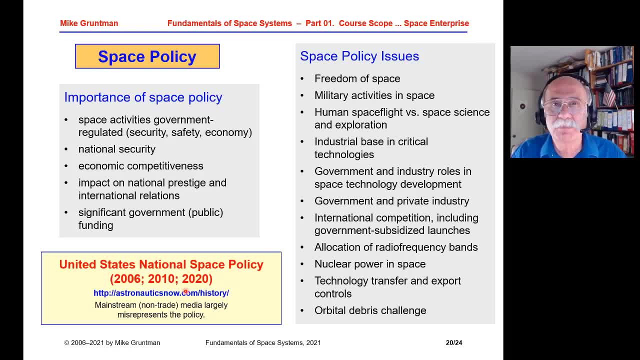 president trump issued his policy. when the space policy is made public, usually in the mainstream media, you can't really understand or learn much, because either journalists are lazy or uninformed or combination thereof, and the political biases and all that it's. it's really misrepresents the 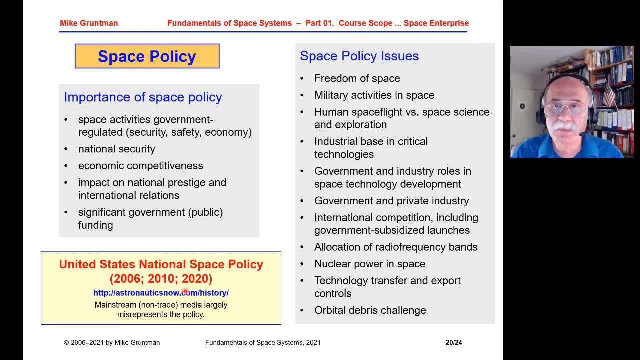 policy some. perhaps laziness plays the most important role there, but the trade media, such as the aviation weekend, space technology, space news, aerospace america, awa's publications usually very good and you will just learn what is there. there are many space policies issues of importance, so, for example, i listed on the right some of them. so 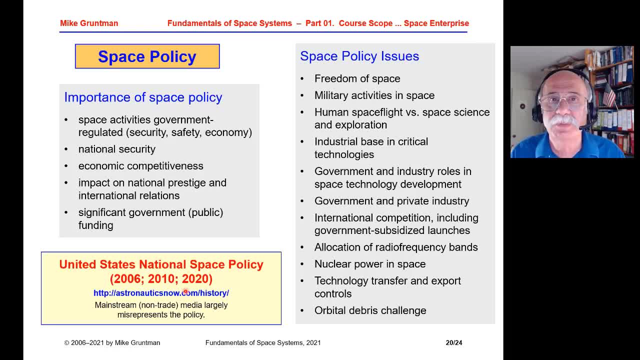 freedom of space is basically: can you fly over other countries territories, can your satellites fly over? today it's no questions, they can. but in the beginning of the space ages was the main, one of the main issues and the questions: military activities of space. we cannot even agree what military activities are. so because, again, everything. 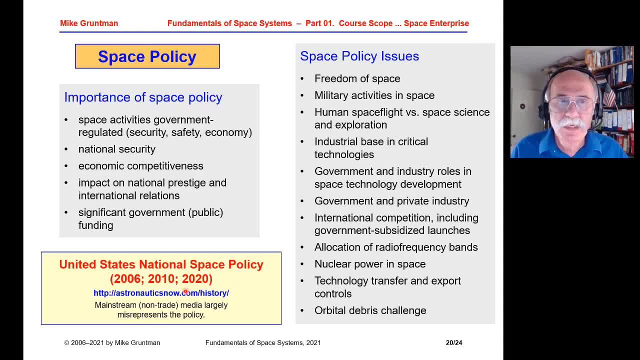 is just so, so combined in the science and technology: the human space flight versus space science and exploration. the tensions between the human space flight, or proponents of the human space flight, and the robotic science exploration were from the day one of the space program in the united states, from the day one from the late 1950s. 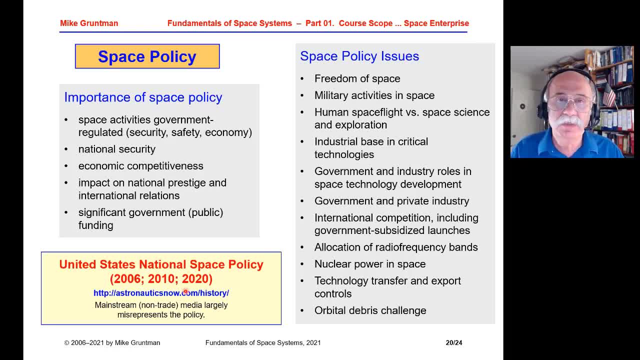 and early 60s, and it continues. you hear the calls of the calls. while we don't need the international space station, let's spend money on science. and if you but a lot of public support comes because of the human space flight for government space, uh, it's again the space scientists and 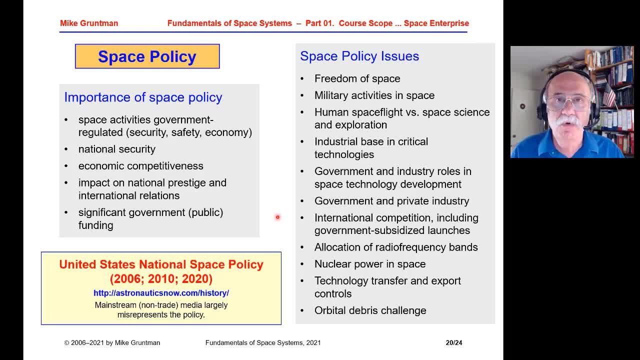 engineers should really be more careful in what they say publicly, because if we get into the too much of a fight among ourselves, we can lose support of public and we will lose both. then industrial base and critical technologies. this is a very important issue because how much government should do in space? because we would like to. 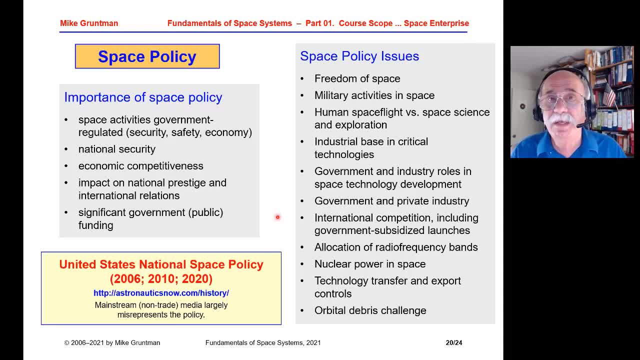 have private companies to produce, to do things. on the other hand, certain technologies that are essential, indispensable for space, they are not very profitable and the companies would rather do things in the commercial world that will bring profit, in the commercial world. that will bring profit and that's why the government needs them to do it. for example, 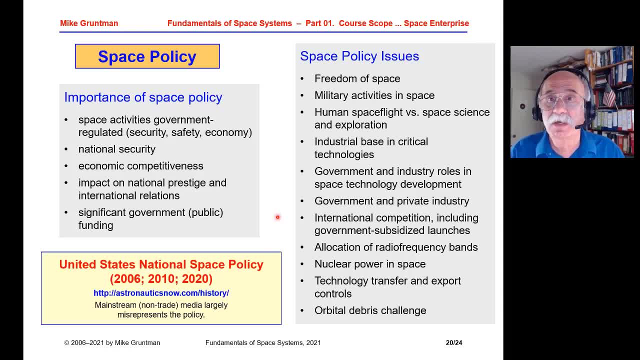 radiation hardened circuitry, integrated circuits that could operate in space, radiation hardened or solid rockets with large diameter that is needed for, for example, for the icbm's launch from submarines or from silos. and if you do not continue these developments in industry, you may lose uh. 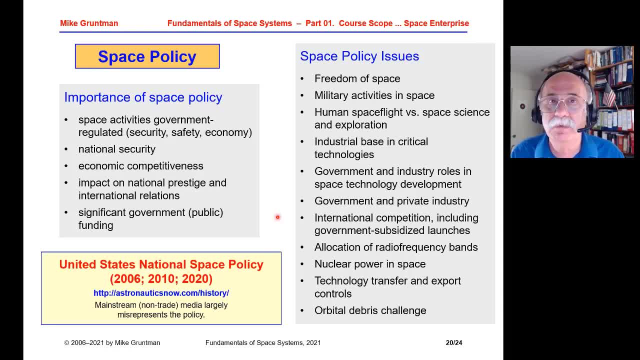 the technological expertise, because you cannot learn many things in textbooks. you have really to pass the experience of one generation of engineers to another and if you don't have the programs r d, research and development programs in certain areas, then sooner or later you would lose expertise as the people retire. 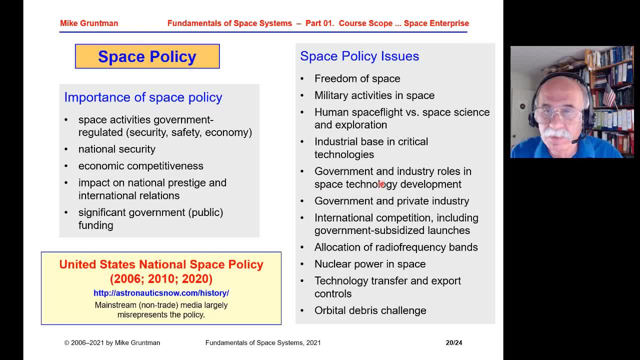 again, industrial based and critical technologies. the government and industry role in space technology development. we already mentioned that um its interaction between government and private industry. international competition, how much we should compete, and is this competition fair? one have to say, one has to say that practically no space launcher was ever. 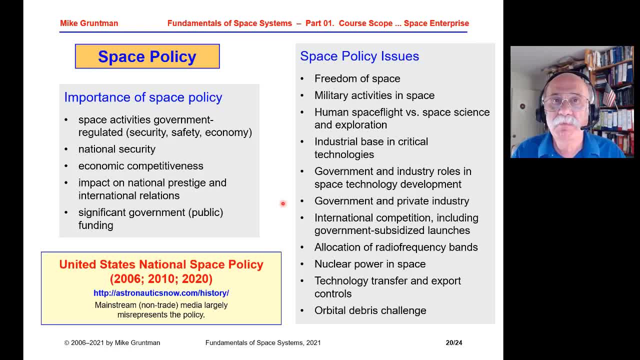 developed until very recently purely commercially. there was a government subsidies in all countries in different shapes and forms. so you have to be just careful when you call for the open competition, because the competition very rarely is open. allocation of radio frequency bands, nuclear power in space technology, transferring expert controls are very 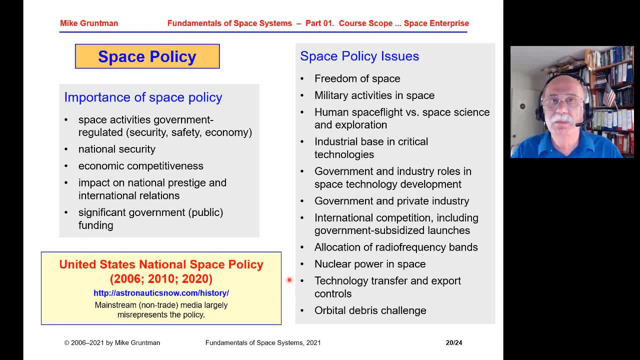 important from the national security point of view and orbital debris challenge. this is something a growing problem, so we have more and more stuff flying there and we will talk a little bit more about that in the space environment part of the this course. if you look at the space mission any, 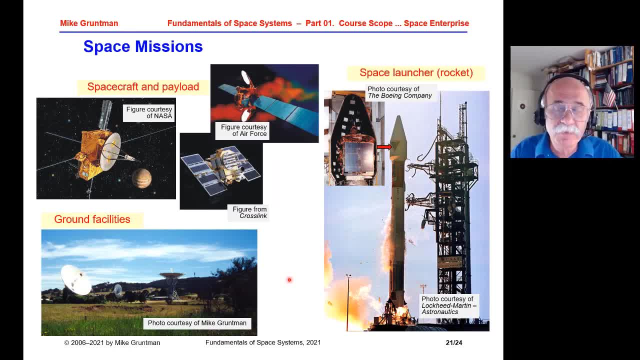 space mission. there are three components. first of all you have to have a payload, a sensor or something that does useful thing in space: either measure certain particles, fields, or take pictures of astronomical objects, or maybe looking down on the earth for remote sensing or reconnaissance or doing something. there is a. 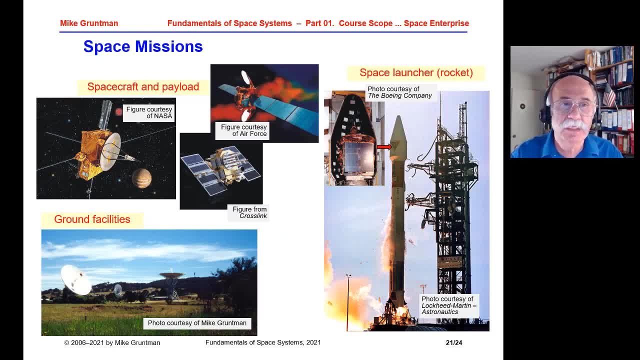 payload, then you need a spacecraft- sometimes called a space craft bus, on which this payload flies, and the spacecraft bus provides a structure. it provides resources, power, communications capabilities, orientation control and all that to a payload to operate. you need a spacecraft and payload and you deploy them in space. then you need the ground facilities, as 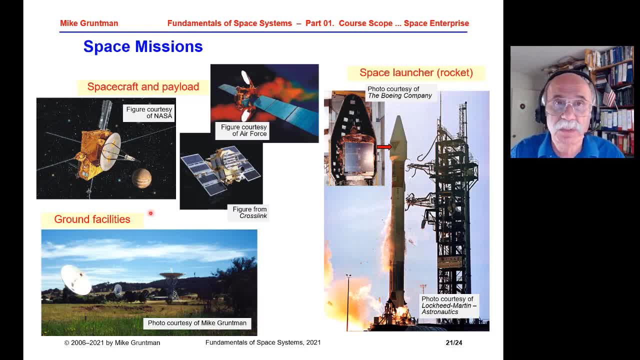 on the ground that would interact with your spacecraft, communicate, control it and, as we saw in the economic part of this of the data just a few minutes ago, this ground infrastructure is very expensive. it just takes a lot of expenditures, significant part of the space enterprise. and then the third main component is space launcher. so you build the 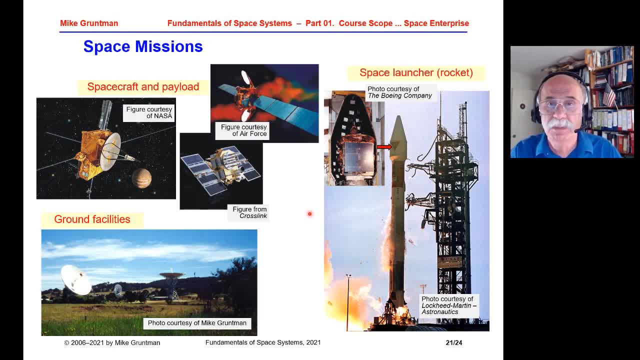 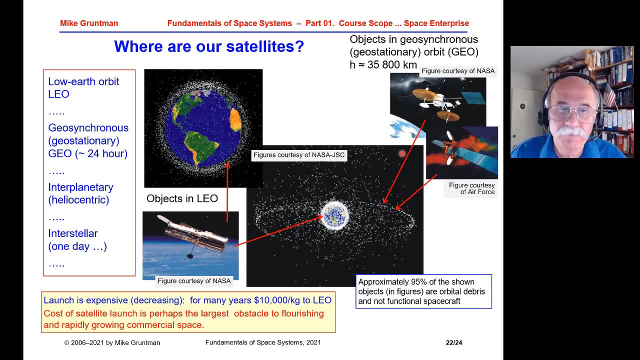 spacecraft and the payload, and in order to deploy an orbit you need a huge rockets and there's space launches that will put your spacecraft into order. these three main components always in space missions. so another question is: where are our satellites? most of the satellites are in the so-called low earth orbit. 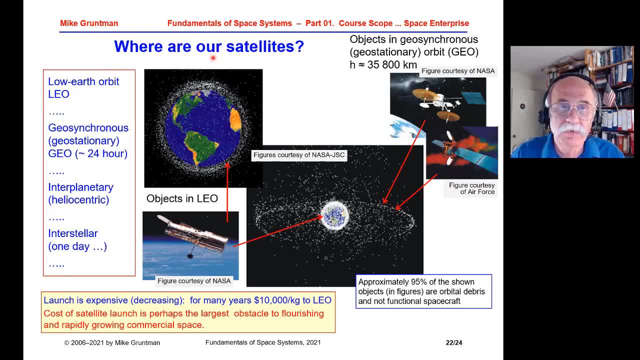 leo. this is a view just shown here of our earth to scale, with the most of the satellites and they are in the lower earth orbit and they are in a shell. you could think about this: about 1000 kilometers or six or seven hundred miles thick earth diameter is roughly 12 000 kilometers. this is to scale. 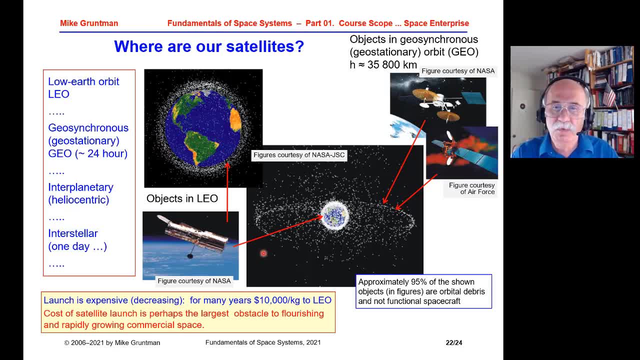 most of the satellites are there. if i step away from the earth and i look, as shown just right here, i would see that, in addition to a satellites around the earth, lowest orbit is a ring of satellites, and this ring of satellites would be at altitude 35 800 kilometers. 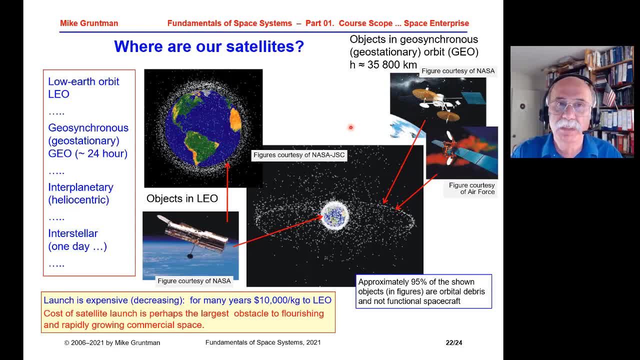 this is the so-called geostationary orbit. a satellite in this orbit appears stationary for observer on the ground. it basically revolves around the earth, uh, with the same rate as the earth's spins on its axis. so we'll talk a little bit more about that in a few minutes. 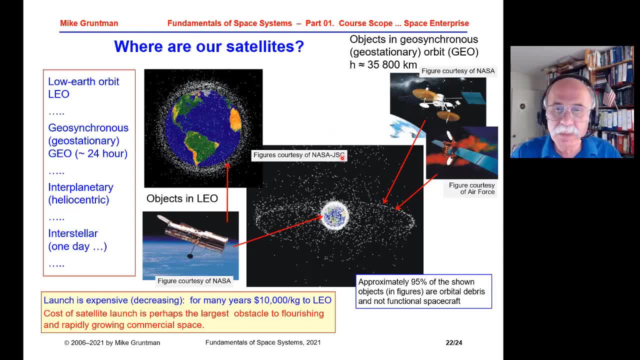 we'll talk in the orbital mechanics more about that. this is a geostation orbit. this is where most of the satellites are low earth orbit and some in the geostationary orbit and of course there are a few satellites on interplanetary trajectories that going to other 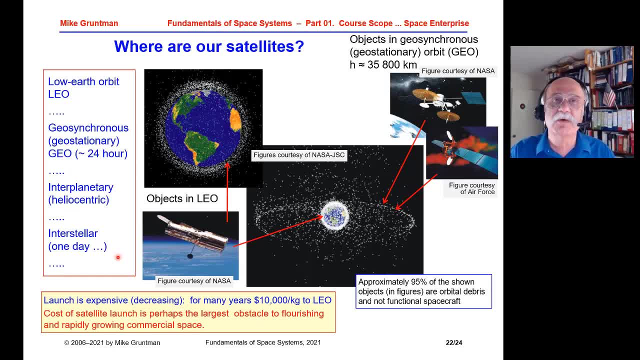 planets for exploration and one day we'll have an interstellar craft leaving our solar system. a launch is very expensive and for many years the cost of launching, say, one kilogram to low earth orbit was about ten thousand dollars. now the launch cost is decreasing. this is the phenomenon of the last several 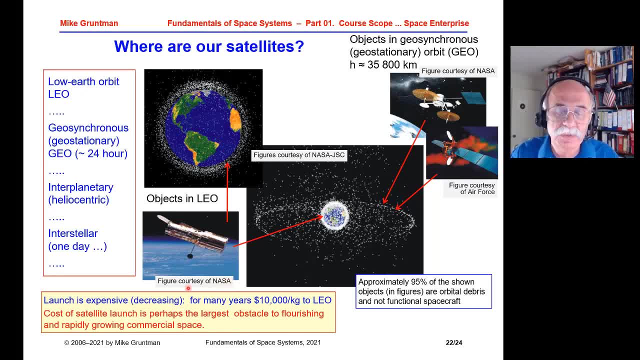 years, there's a growing competition among various space launches. space x also contributed to to changing uh the way how the business is being done. so the cost is exp decreasing but it's still very expensive, and the cost of satellite launch is perhaps the largest obstacle to flourishing in a rapidly growing commercial space. 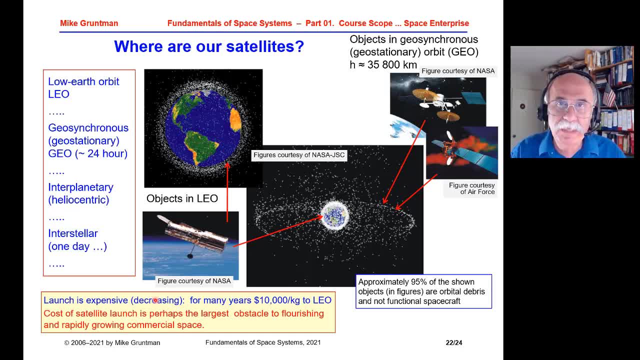 although now the commercial space is gross, the cost is going down and we will see more and more of these tendencies. as the cost of the space launch becomes smaller and smaller, there will be more and more activities in space and there will be more and more challenges with debris. 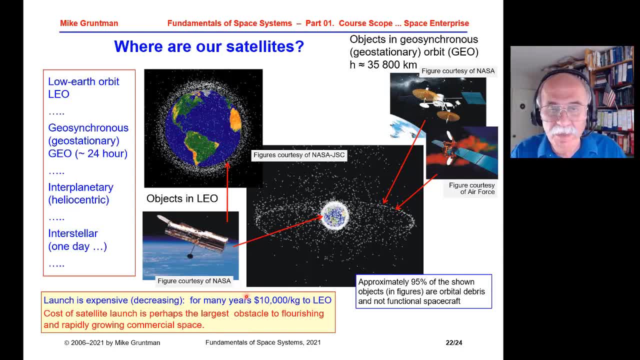 problem. but anyway, the uh keep in mind this number for the rough estimate. so for many years it was ten thousand dollars per one kilogram to place in the lowest orbit. and uh, today, just it's a little bit, just a little bit. and uh, today, just it's a little bit, just a little bit, just a little bit, just a little bit. 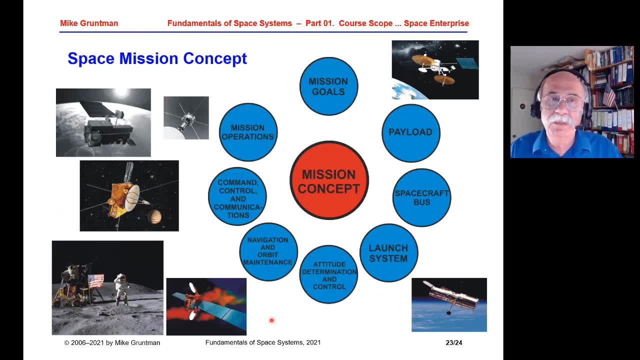 lower. if I look at the space mission concept, everything is driven by the mission goals. very few cases now when the countries fly just a satellite to show the flag, just for the prestige purposes for the big countries it is in the past. today we fly spacecraft to do something in space, to do remote. 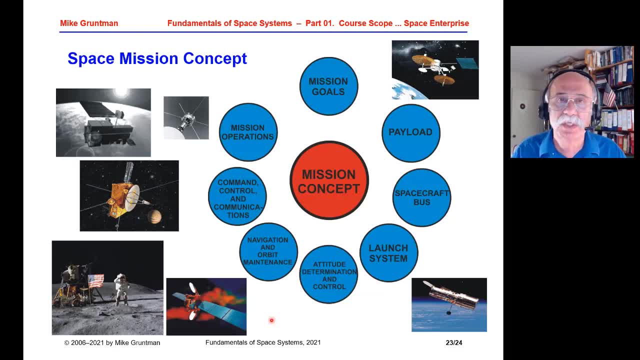 sensing some military activities, communications, or to to perform particular scientific measurements and exploration. there's a mission- goals is something that drives the mission. so in order to achieve the goals, we have to have a payload that would on board of satellite that would achieve this mission goals. then we have to have the spacecraft. the spacecraft. 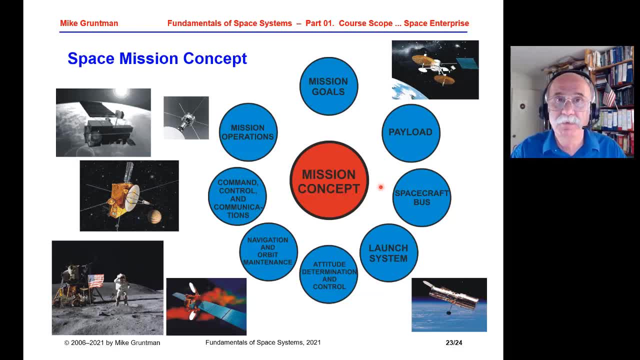 but, as we already introduced this term, basically payload rides on the bus, and the bus provides all the resources for the payload to operate. now we also have to have a launch system to put our spacecraft into the right orbit to achieve the mission goals. and when I am an orbit, I need attitude determination. 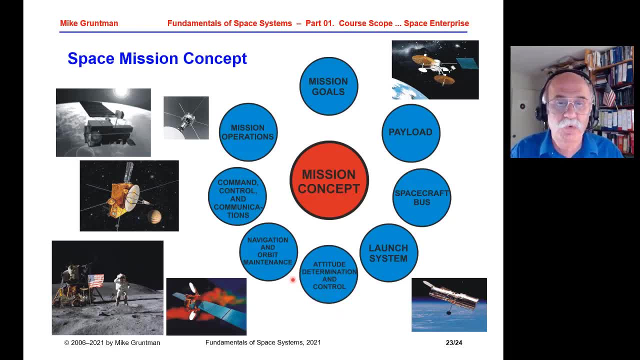 control and again we will be discussing it later in the course. we have to navigate and maintain the orbit. we'll discuss it later in the course. we have to have a command, control and communications capabilities and we need to power our spacecraft and we need to provide thermal. 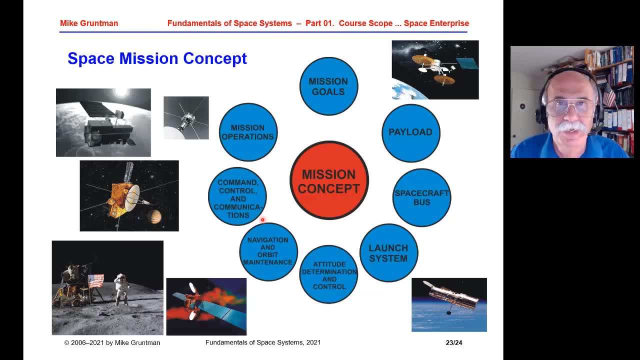 control there. so well again, we'll be discussing this during our course later. and then, finally, we have a very important component: mission operations. mission operations that will control the spacecraft during the mission, receive the data, store them and distribute to the users. and there's number of the beats coming from space growing dramatically. it's 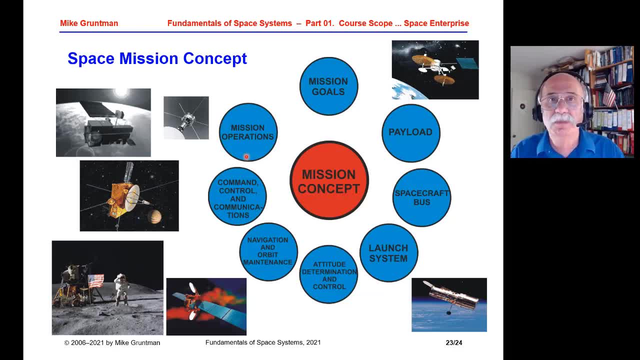 takes more and more effort to do that. and then you have to control the spacecraft from the ground. all these components have to be tied up together in order to have a mission that would successfully achieves its goals. the system engineering becomes very important because many areas of science